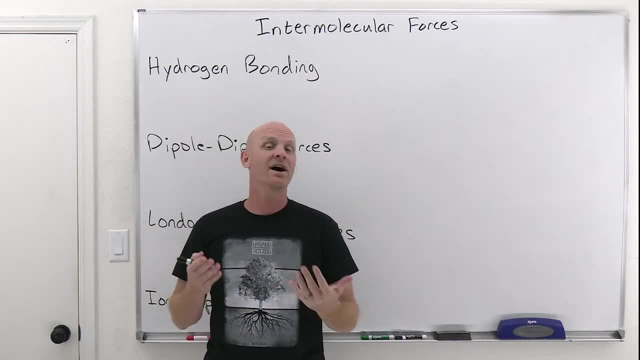 it turns out all the ions are held together by ionic bonds in an ionic solid, So in a network covalent solid, like you know, a diamond and things of a sort. So again, all the atoms in that diamond are held together by covalent bonds. Well, it turns. 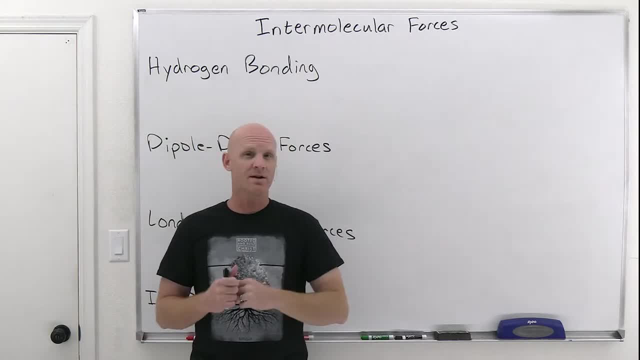 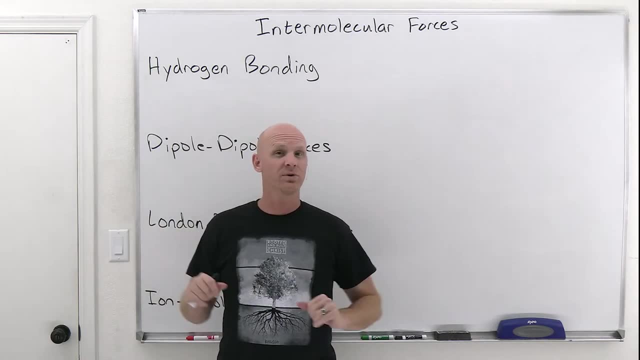 out when you've got molecular compounds and whether you're, you know, like I said, we're talking about a molecular solid like ice. Well, it turns out what's holding those molecules together? So, and again separate molecules, again you might have the individual molecules. 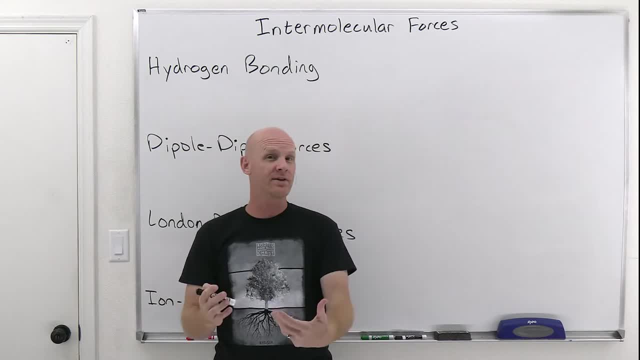 are held together. The atoms within one molecule are held together by covalent bonds, but if you have a molecule over here and a molecule over here, what's actually causing them to you know? stick together in the ice crystal, if you will, is something much weaker than an. 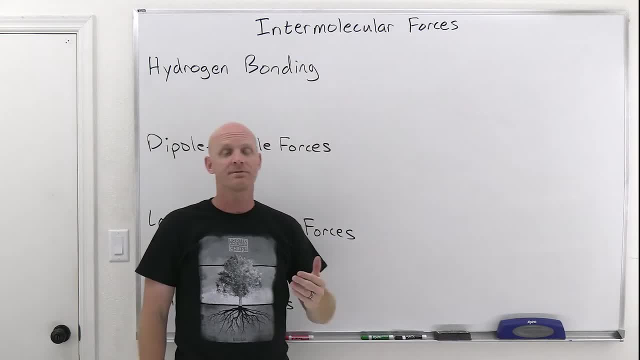 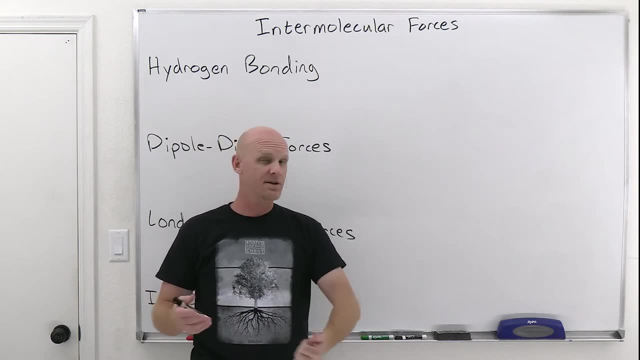 actual bond, which we call these intermolecular forces. And so, first off, you should know they're way weaker than an ionic or covalent bond like, on the order of like 25 to 100 times weaker, So significantly weaker. So, as a result, these molecular compounds tend to be held together. 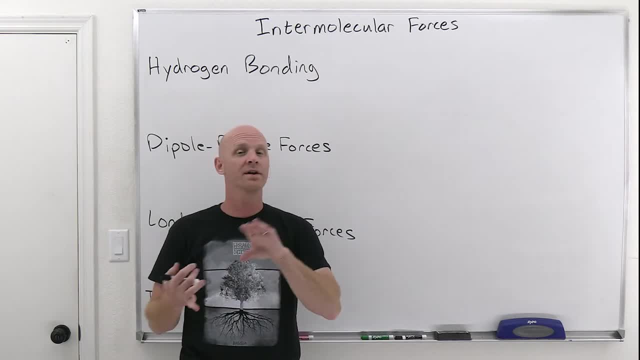 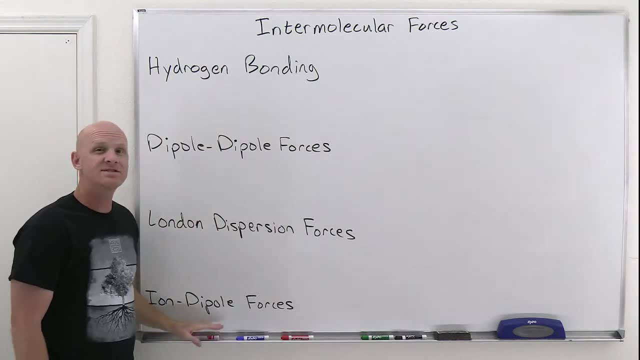 if you will, much less strongly than, say, an ionic compound or a network covalent compound. as a general rule, All right. so these intermolecular forces- I'm going to talk about ion-dipole forces at the end. 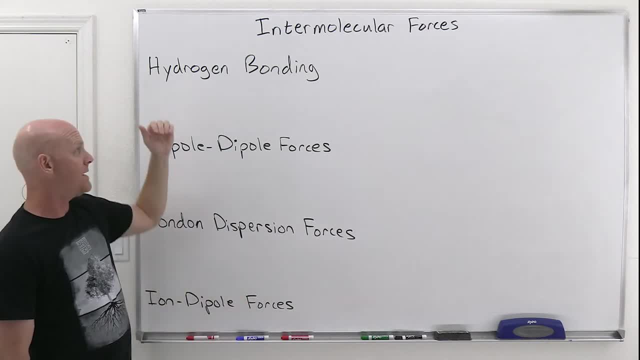 and it's kind of part of a separate discussion and we'll see why. But for hydrin, bonding, dipole-dipole forces, London dispersion forces, we'll talk about these at the same time And in general, as long as you're talking about molecules that are all very similar in size, 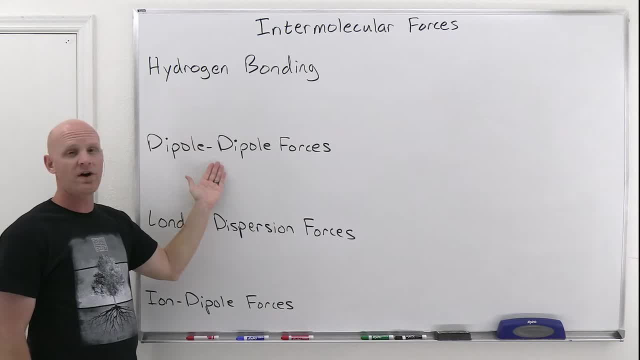 we'll find out that hydrin bonding is the strongest, and then dipole-dipole forces, and then London dispersion forces. So, but if your molecules are not all similar in size, it's going to be a little more challenging. So we're going to go through some of those comparisons as we go. 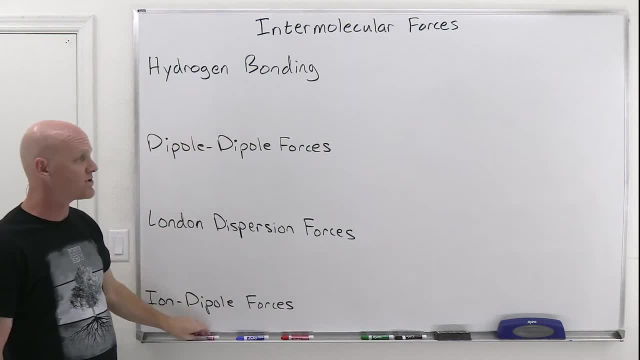 We're actually going to start by talking about dipole-dipole forces first. So because I like to think of hydrin bonding as a super-duper strong dipole-dipole force, so it might be helpful to actually define these dipole-dipole forces first. 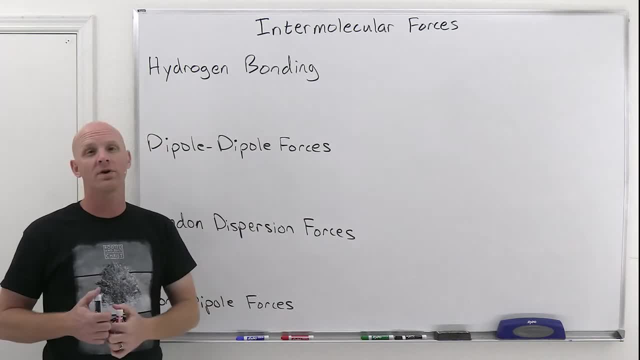 Now earlier in the course here we've learned about polar molecules, and polar molecules have a dipole moment And it turns out that's the requirement for dipole-dipole forces. It is one of the intermolecular forces that's going to be present between polar molecules. 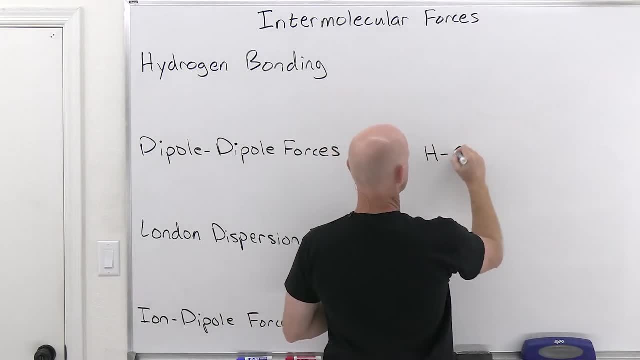 They have to be polar. So my favorite example of this is using something like HCl and HCl here. So hydrin is less electronegative, chlorine is more electronegative, And so there's a big polar bond here. 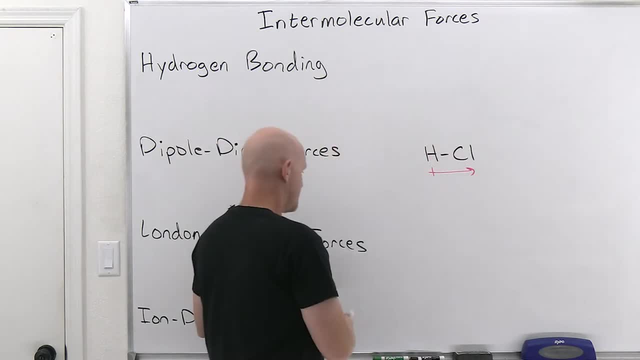 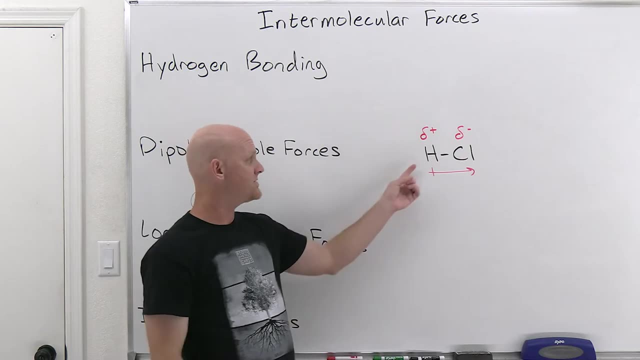 And we could represent that, you know like so. But the other way we can represent that is with our partial positive and partial negative symbols. Now, this hydrin is held to this chlorine through that covalent bond. we represent with a line here: 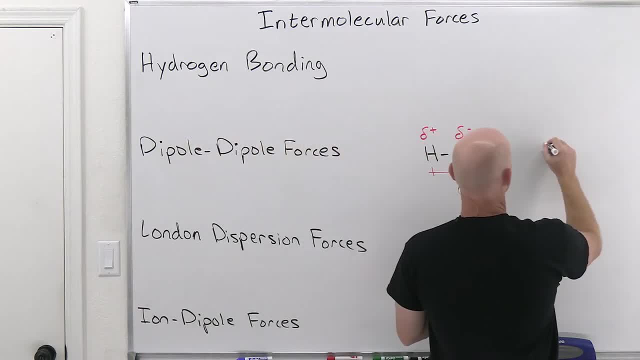 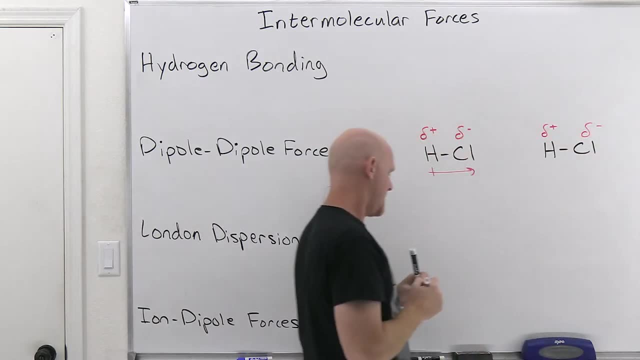 But that's not what we're talking about in this lesson. We've got to draw a second molecule here And again. this hydrin is also partially positive and this chlorine partially negative, And what we're ultimately talking about in this lesson is the attractive force between these separate molecules. 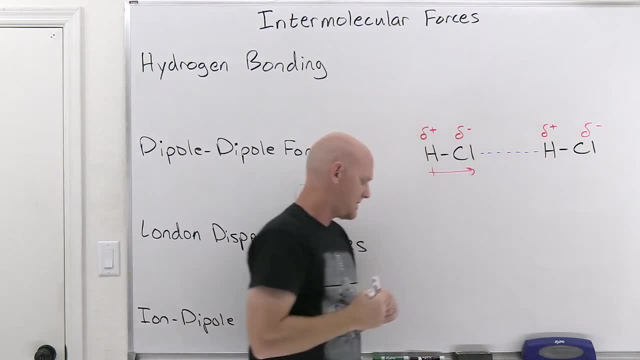 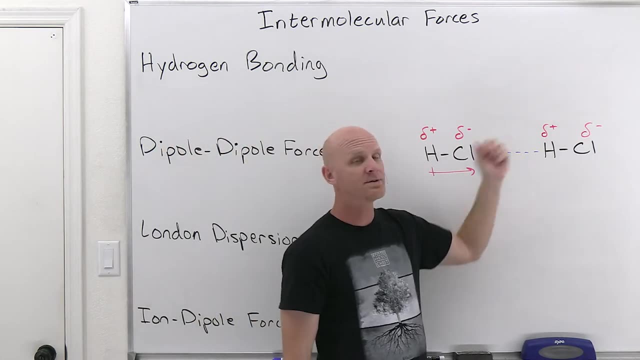 And there is a weak attraction here. And the nature of these attractions is all about plus and minus, And so it turns out this chlorine is partially negative and this hydrin is partially positive And, as a result, there's a weak attraction to here. 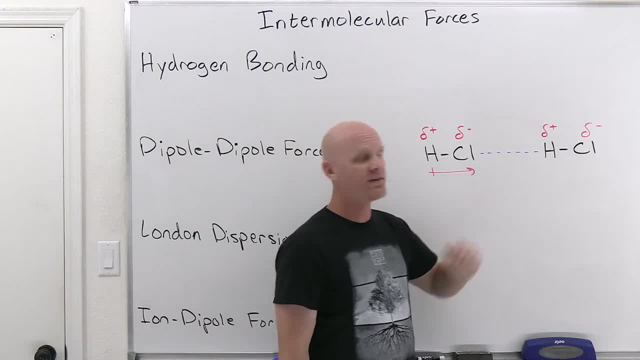 And again, it's way weaker than an actual covalent bond. So again, what holds this chlorine to this hydrin is a covalent bond, a rather strong interaction. So what's the nature of the attraction between this chlorine and this hydrin? 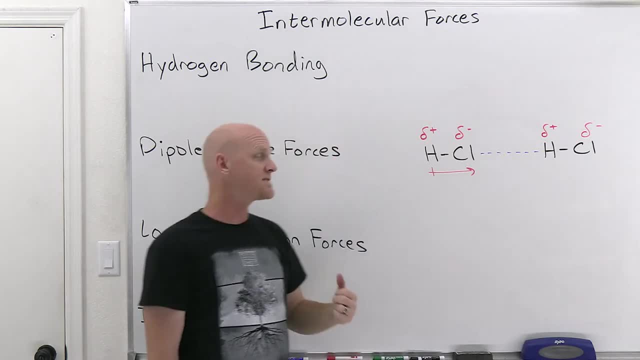 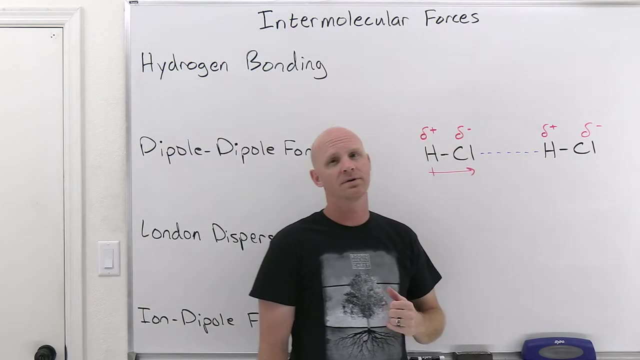 Well, that's an intermolecular force, something much weaker, And in this case it is a dipole-dipole force, And it arises because this molecule has a permanent dipole and because this molecule has a permanent dipole And, as a result, part of this molecule being a little bit negative, part of this one will be a little bit positive. 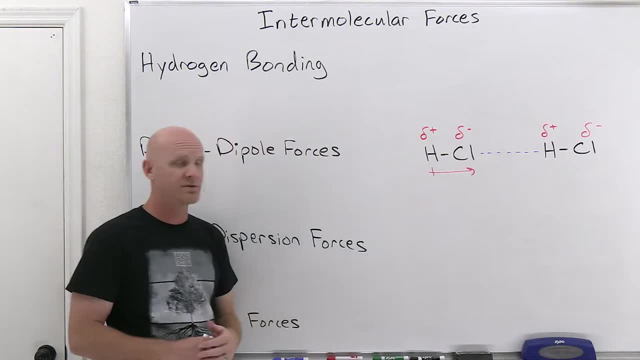 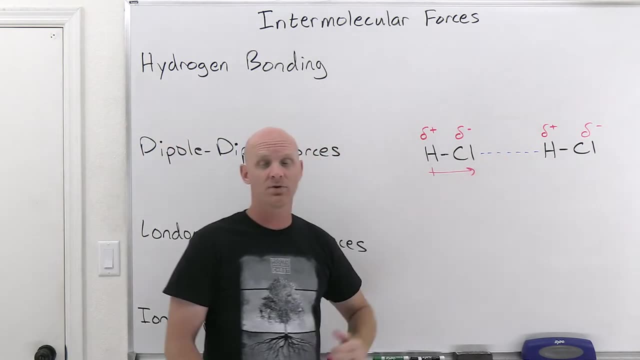 And those are the parts that will be attracted to each other. So that's dipole-dipole forces. Generally, the more polar the molecules, the stronger the force. And here I show it for two identical molecules, like if you had pure HCl. 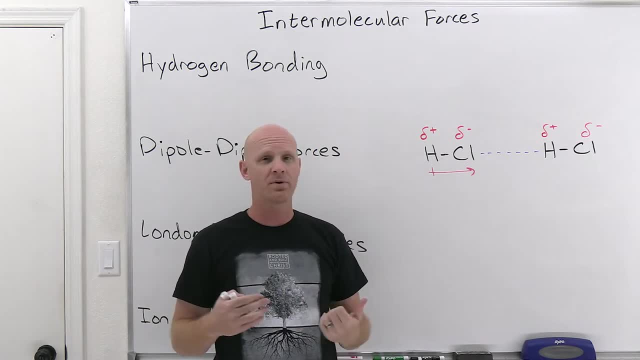 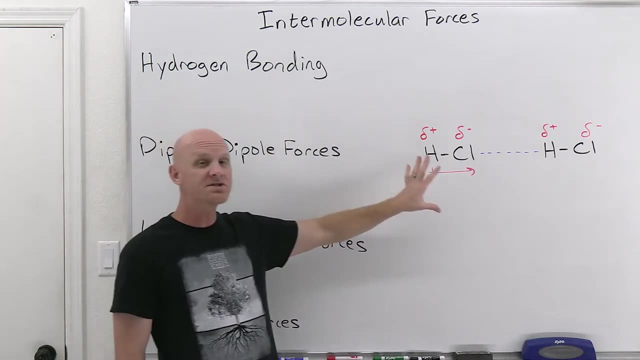 But if you had a mixture of polar molecules, again, they all have to be polar, So then you could also still have these dipole-dipole forces interacting. Now we'll find out. it's going to be instructive to consider pure substances. 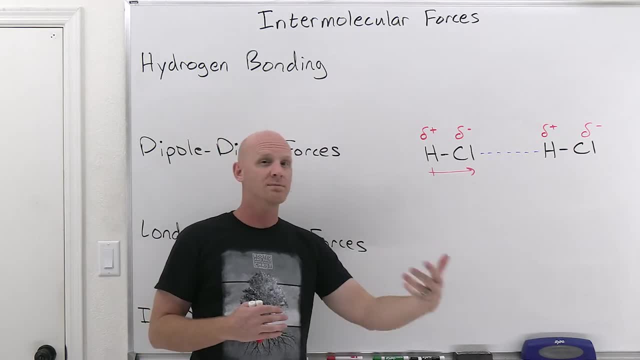 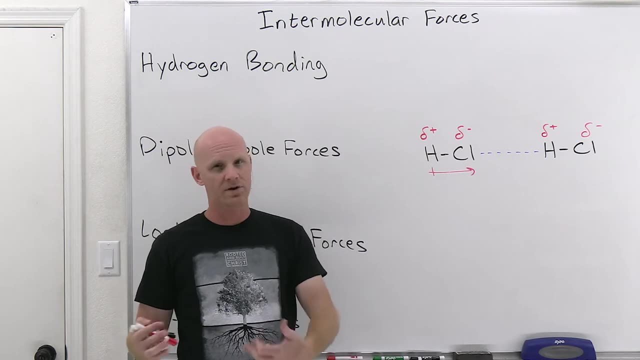 because that's when we'll talk about, like ranking boiling points or ranking melting points, or comparing viscosities or surface tensions, vapor pressures, things of this sort. So, whereas for a mixture you wouldn't normally compare those things, But you can still talk about what kind of intermolecular forces. 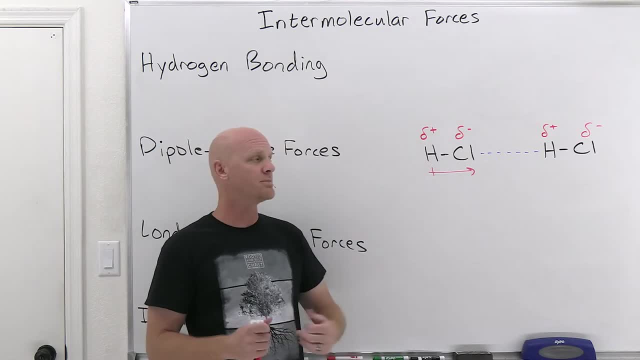 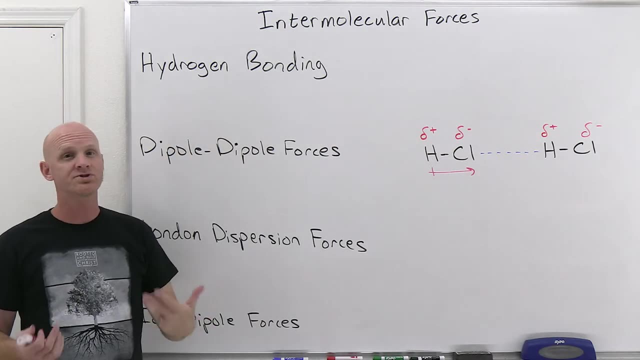 are present in mixtures. We're just not going to then apply it usually to the some of the bulk properties of those liquids. All right, so hydrogen bonding, it turns out, is kind of like a super-duper strong dipole-dipole force. 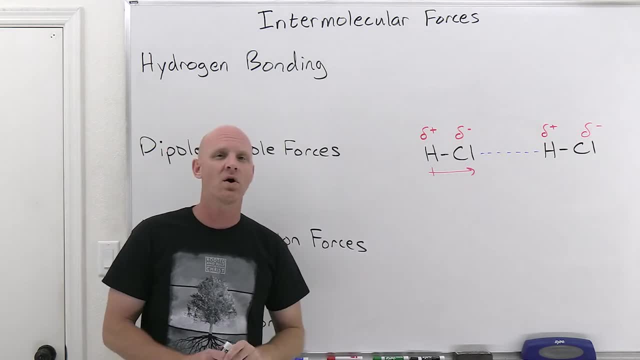 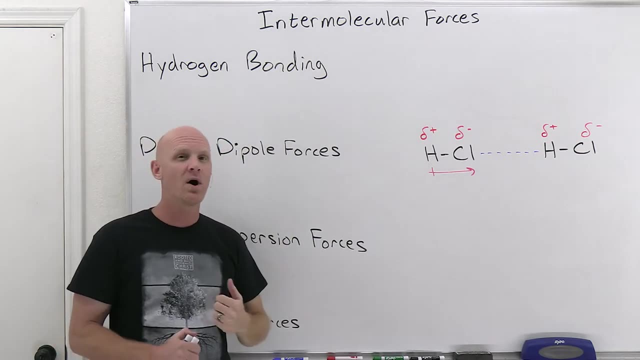 So, but it turns out there's only three different kinds of molecules that are going to have these super-duper-duper strong dipole-dipole forces that we call hydrogen bonding, And it turns out that the bond dipole you have to have is always going to involve hydrogen. 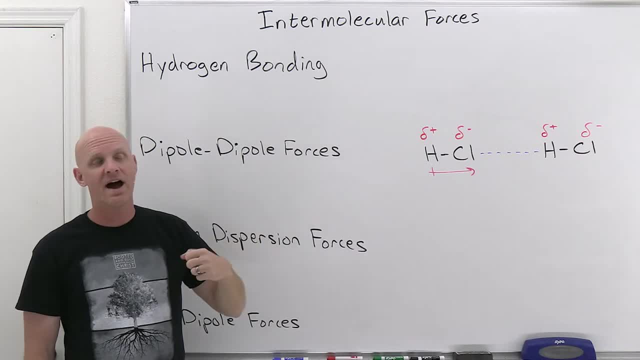 And that's kind of where the name comes from. But it turns out having a hydrogen atom is not enough, because lots of molecules have a hydrogen atom and they're not capable of hydrogen bonding. It turns out that that hydrogen atom has to be bonded to one of three small and very electronegative atoms. 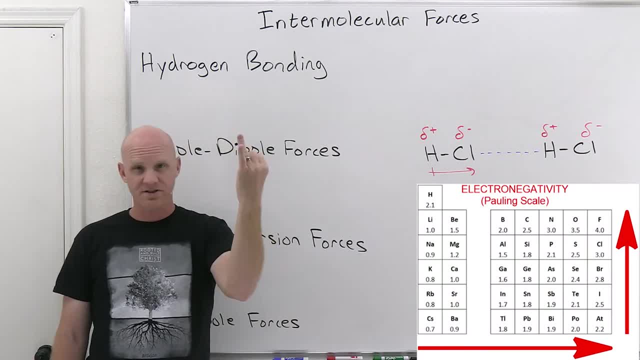 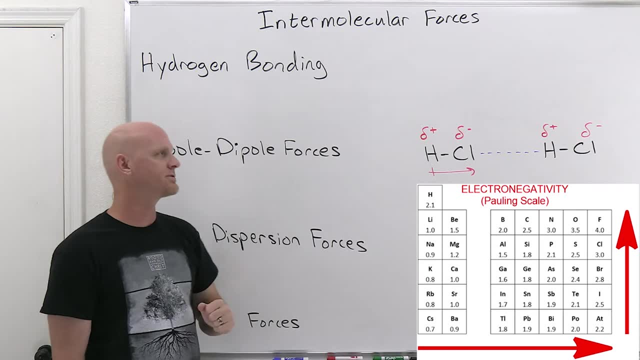 So fluorine, most electronegative element there is, Oxygen, second most electronegative element there is, And then nitrogen, which is kind of in the running for being the next most electronegative, depending on what list you consult and stuff. 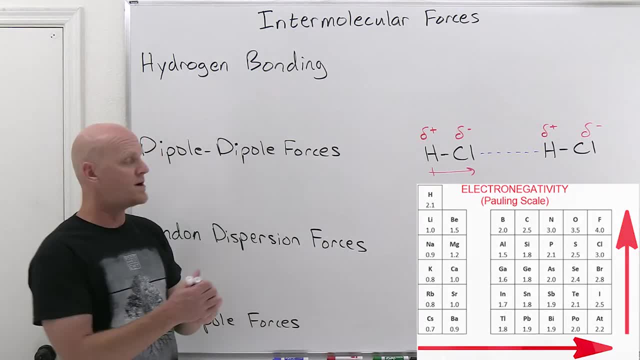 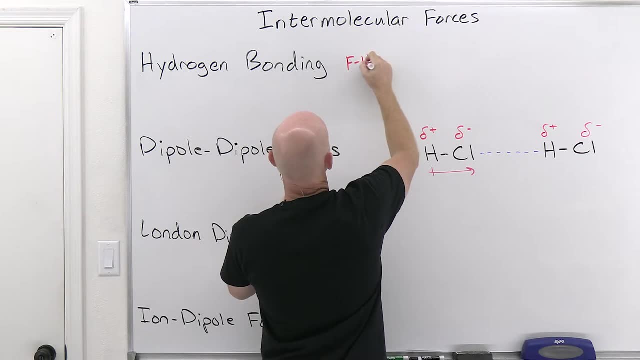 So. but it turns out, if you have a hydrogen bonded to either an F, an O or an N, so then that molecule will be capable of hydrogen bonding, And so in this case we need again an FH bond, an OH bond or an NH bond somewhere in the structure. 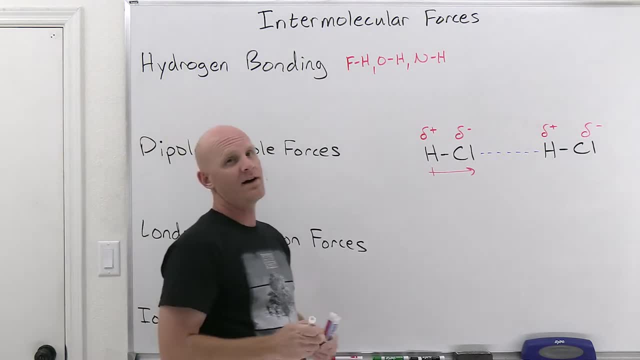 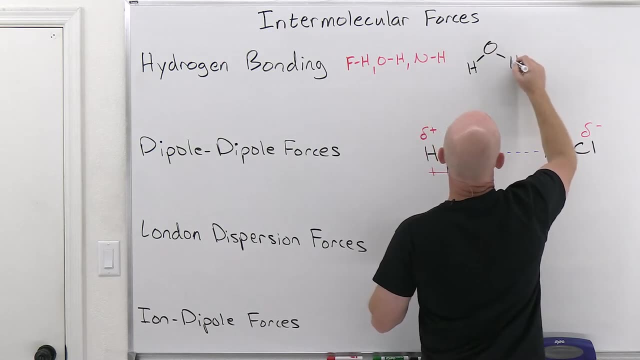 to be capable of hydrogen bonding, And the most common example is that you're likely to encounter every day of your life is water, And so we take a look at a water molecule here. We'll draw two of them, And same we have like with HCl here. 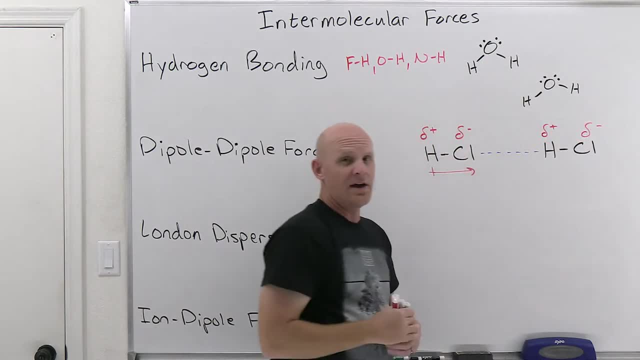 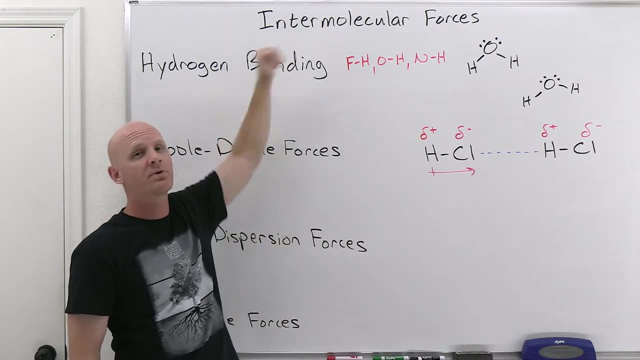 So you've got the partially negative oxygens, the partially positive hydrogens And again the interaction. here it turns out it's so much stronger than anything else we classify as dipole-dipole forces that they put it into its own separate category. 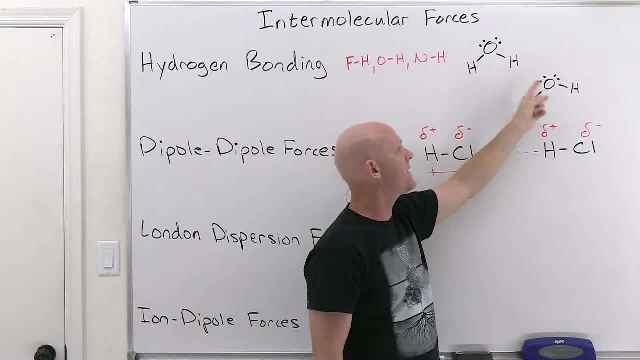 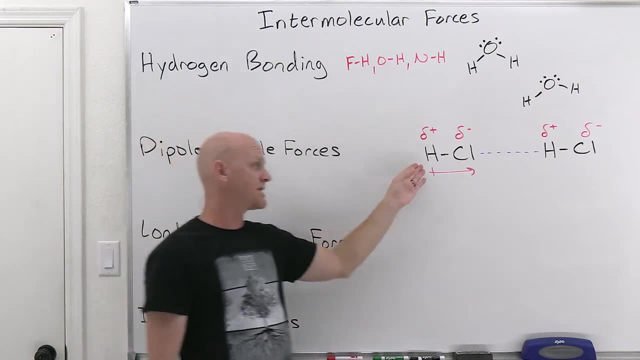 So it turns out these hydrogens are so partially positive that the interaction between the partially negative oxygen and the adjacent molecule here is stronger than all the other dipole-dipole forces that we could see with, like HCl and things of this sort. And so when you've got one of these three very, very, very polar bonds, 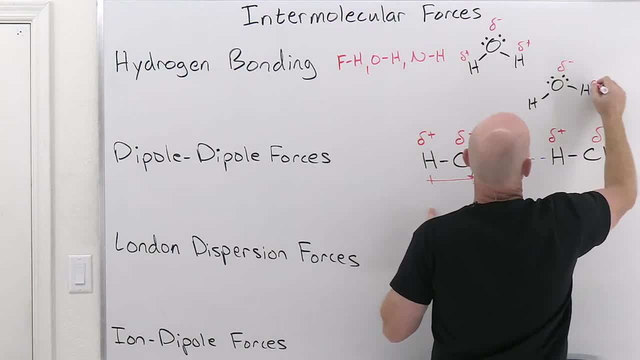 the amount of partial positive and negative is so high that the interaction is just again so much greater. we give it its own special name here. And so in this case it turns out you actually. it is mediated through that lone pair of electrons, And so the lone pair on the partially negative oxygen, fluorine or nitrogen. 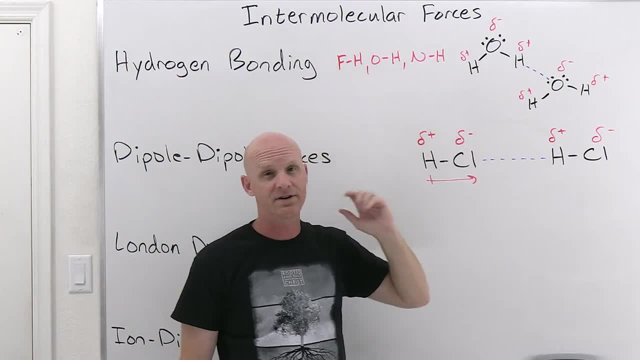 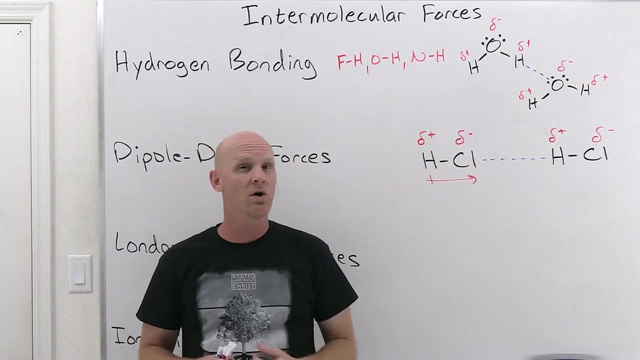 is going to interact with a hydrogen. But again, it can't just interact with any hydrogen, It has to be a hydrogen. that's really partially positive, because it itself is bonded to a fluorine, an oxygen or a nitrogen. Cool. So the atom that has, or the molecule that has, the fluorine, oxygen or nitrogen with lone pairs. 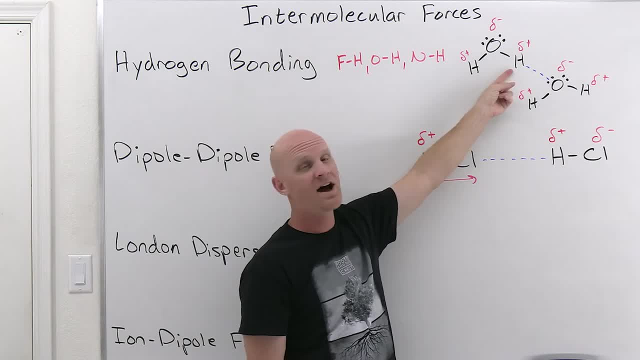 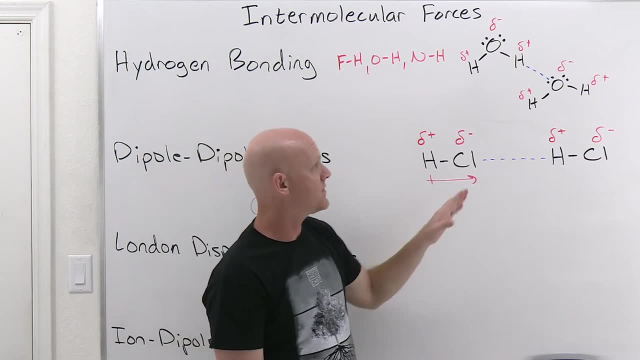 we call the hydrogen bond acceptor, And then the molecule that has the hydrogen, that's involved in the interaction, that's bonded to a fluorine, an oxygen or a nitrogen, is called the hydrogen bond donor. And so in this case you can see that every water molecule has two lone pairs on the oxygen. 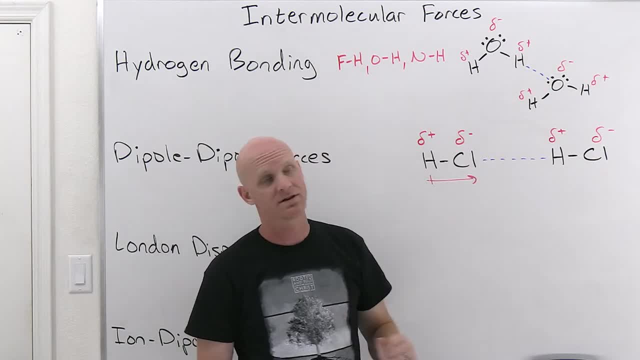 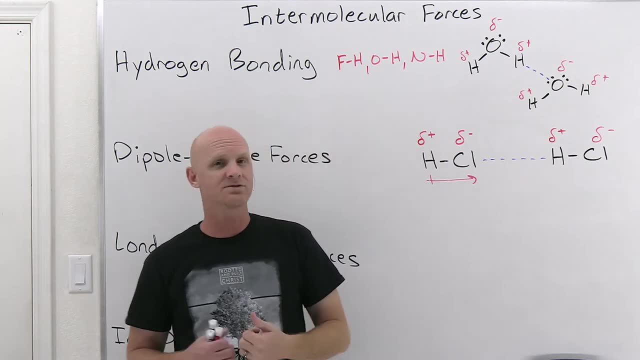 and so could act as a hydrogen bond acceptor up to two times. And each water molecule has two hydrogens that are bonded to an oxygen, and so could act as a hydrogen bond donor up to two times as well. And so it turns out in liquid water. you know, every water molecule has a chance to be interacting. 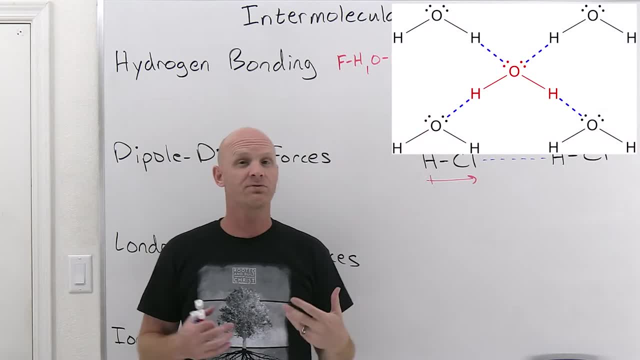 with up to four other water molecules. In fact, when you freeze ice, you do have every molecule interacting and surrounded by four other water molecules, Whereas in liquid water it's somewhere, on average, between two and three, And so it turns out to go from liquid water. 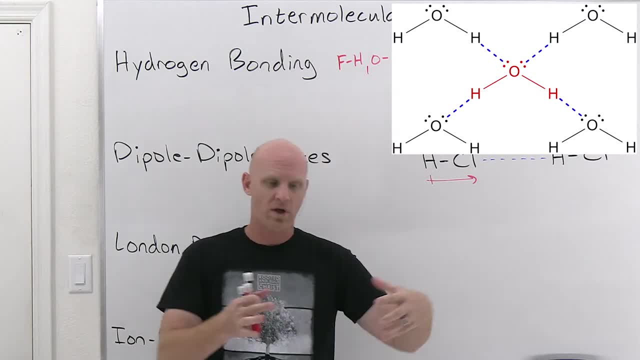 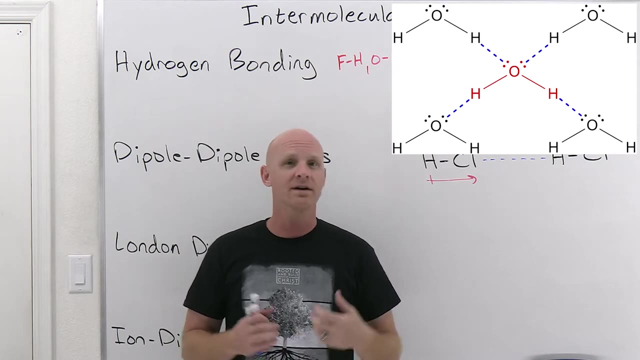 to ice. so the water molecules actually have to spread out a little bit to fit that perfect crystal structure where every water molecule gets to interact with four others, And that's why when you freeze water it expands in forming ice, whereas for almost any other substance you could ever name. 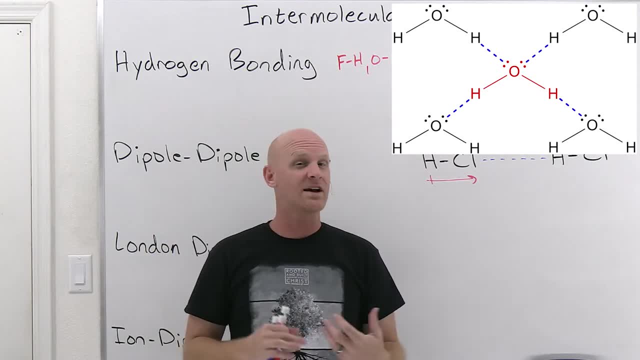 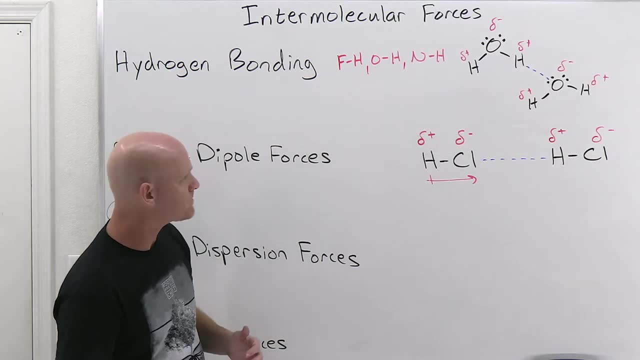 so when you go from a liquid to a solid, it actually contracts and gets smaller. That's actually rather unique for water, So we'll address that and speak about that again in the next lesson and talk about what's special about that. Okay, so if you look at something like say: 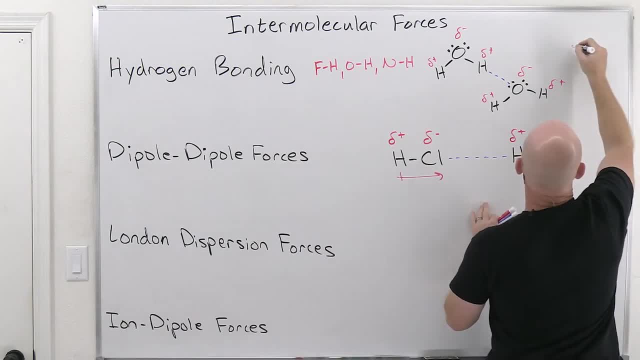 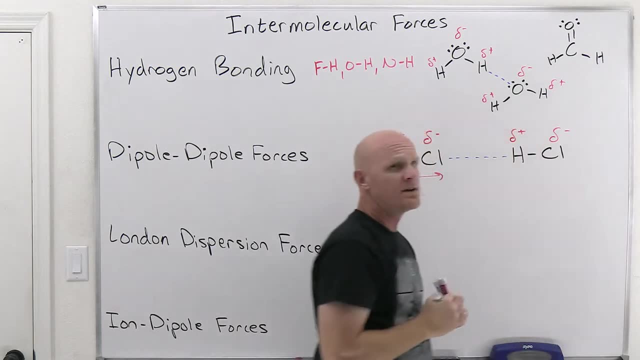 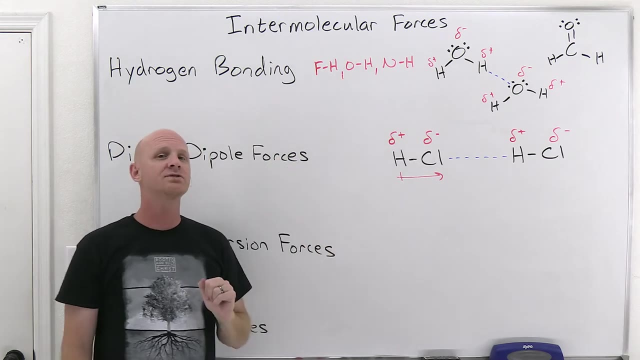 let's go with formaldehyde here. So I just want to give you an example of a molecule here that has H's and has O's, but it does not have an OH bond anywhere in the structure, And so, as a result, formaldehyde here would not be capable of hydrogen bonding. 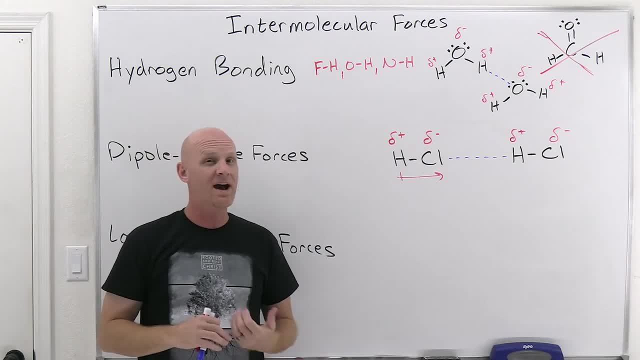 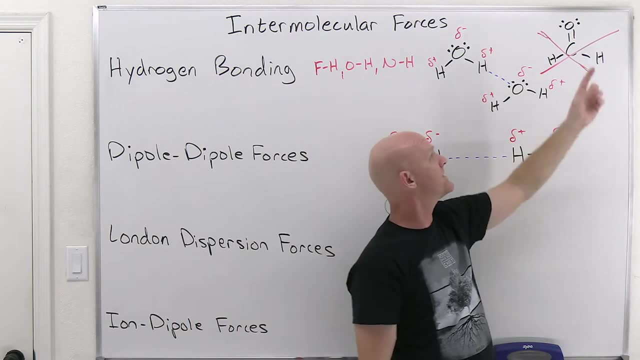 So now it turns out it's a polar molecule. It has a permanent dipole, so it would have dipole-dipole forces, but it would not be capable of hydrogen bonding. And again, a lot of students get lost on the fact that you have O's and you have H's. 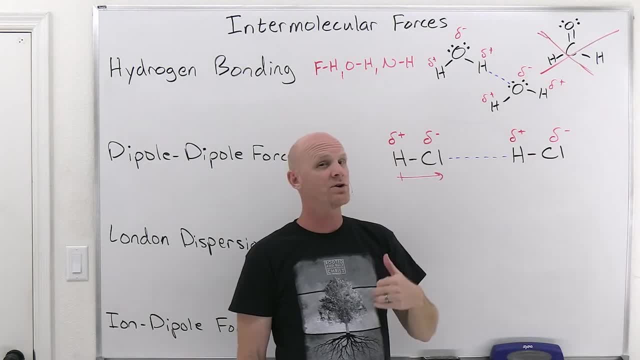 Why not? Well, again, the key is you do have an O, and that's good. That's halfway there. You have a hydrogen bond acceptor right up there. The problem is that these hydrons right here are not significantly partially positive because they're not bonded to an F, an O or an N. 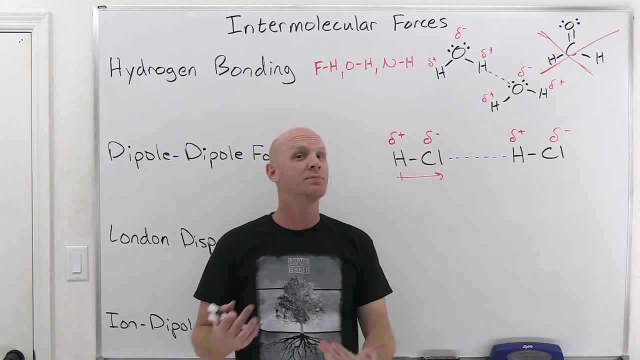 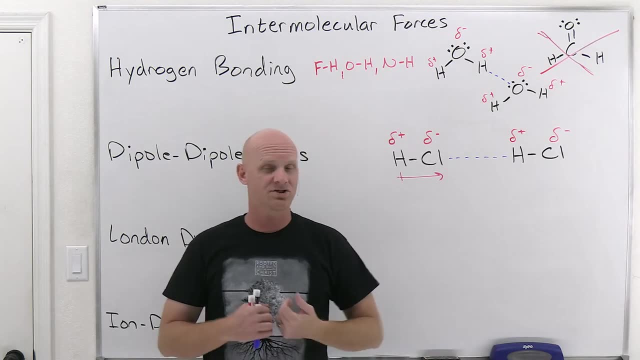 They're bonded to a carbon and, if you recall, we actually consider the carbon-hydrogen bond to be non-polar bond, And so there's no significant amount of partial positive on those hydrons and therefore no great reason why they should strongly interact with an oxygen. 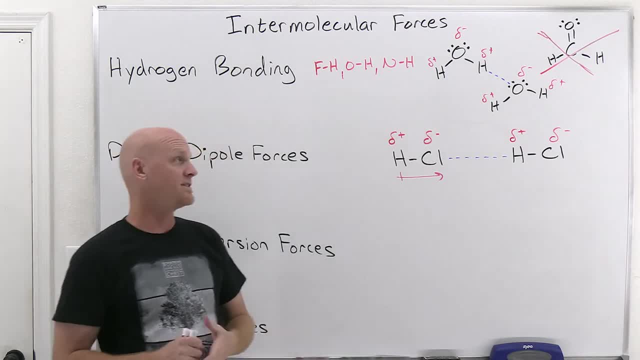 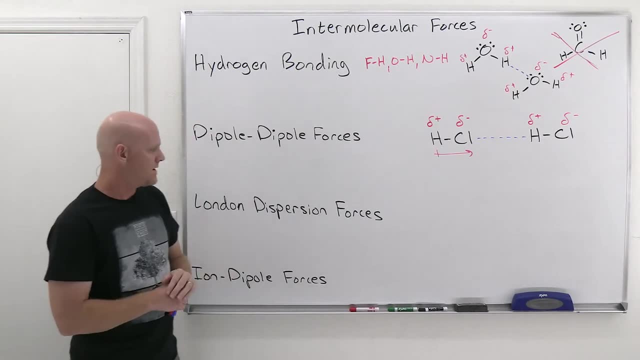 on a nearby molecule in any way, shape or form, So at least not by something we'd call hydrogen bonding, Perhaps by something we might call a dipole-dipole force and stuff, but not by hydrogen bonding. Okay, so now we got to talk about London dispersion forces. 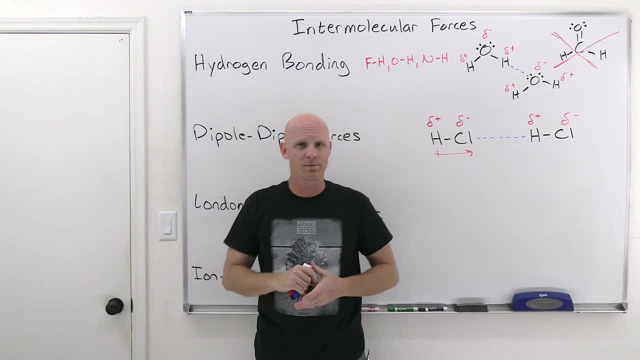 So let's say that you're a non-polar molecule and I'm a non-polar molecule, and so is there any reason we should be attracted to it? Is there any reason we should be attracted to each other? So, based on the discussion we've had so far, it doesn't seem like there is. 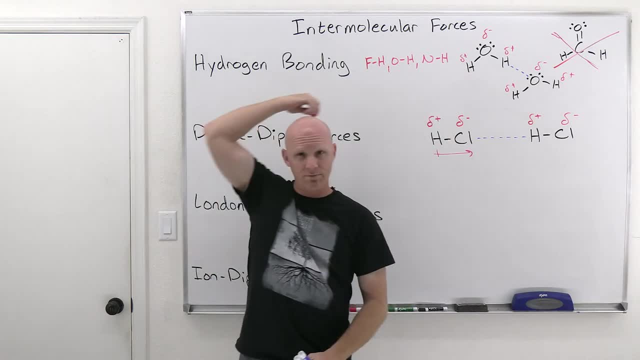 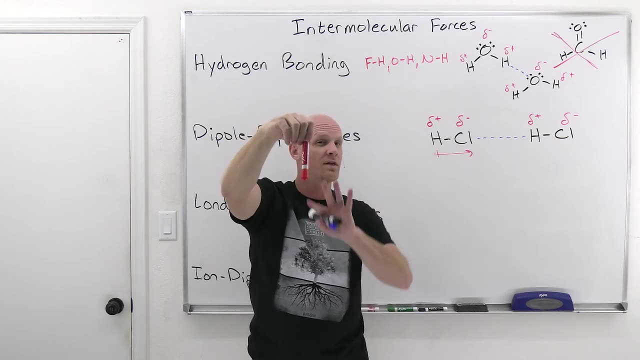 except that my electrons are in motion, So moving around me, my electrons are in motion and we're just going to freeze right here. And so, facing you right now, because my electrons are more on this front side of me, I'm a little bit negative facing you. 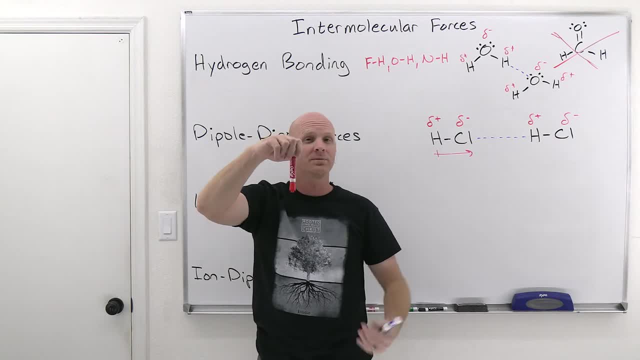 And so what you're going to do is you're going to move your electrons around behind you, and so that, facing me, you're going to be a little bit positive And I'm going to be like dude, we should totally hang out. I never noticed. 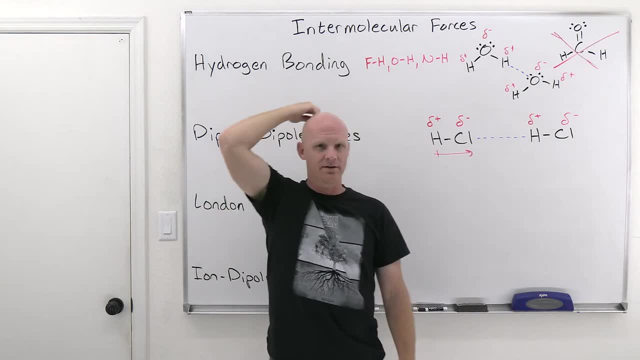 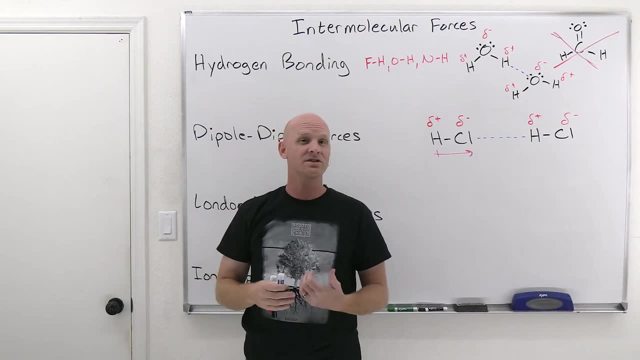 I think we'd hit it off And then my electrons move and I'm like, oh, never mind. So the idea: with a non-polar molecule. they do not have a permanent dipole. however, they can have a temporary dipole just due to the motion of electrons. 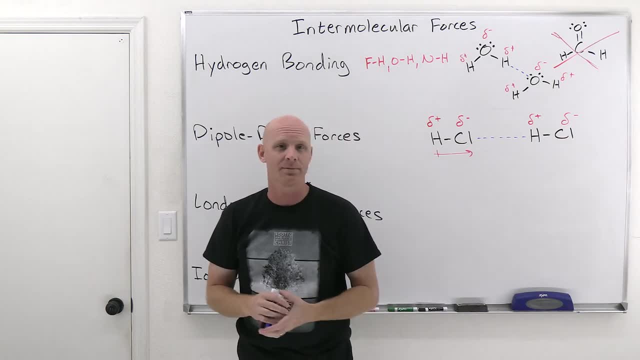 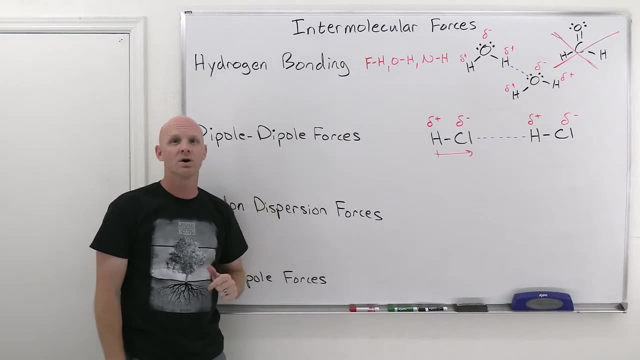 And it can induce the molecule right next to them to also have a dipole. and it turns out that's what we get when we have London dispersion forces. It's just due to the nature that we have electrons in motion And even molecules that don't have a permanent dipole can still have temporary ones. 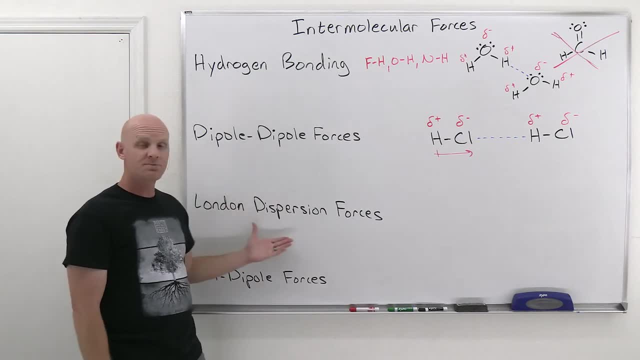 and induce the molecules around them to have one as well. In fact, London dispersion forces are often called induced dipole forces as well. Cool, Now it turns out the thing is not only do non-polar molecules have these, but it turns out all molecules have these, because all molecules have electrons. 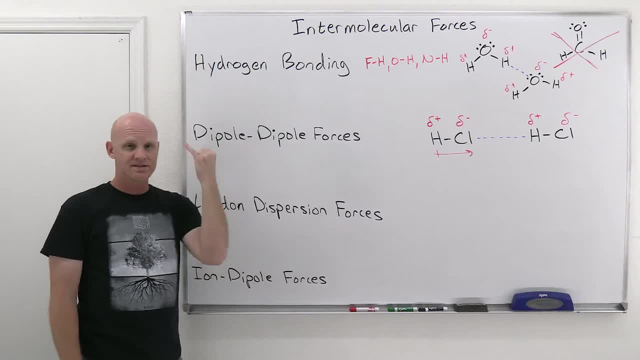 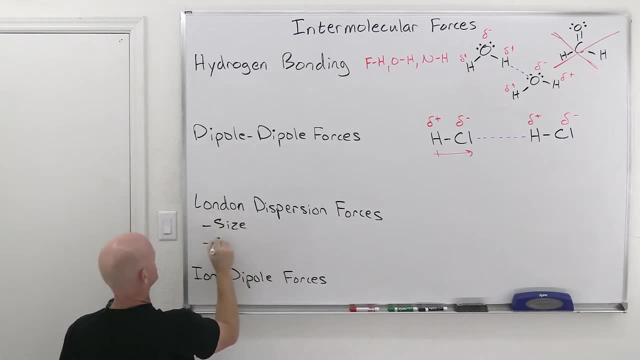 And so, and it turns out they're really dependent on two things: Size and surface area. Let's write that down. And so it turns out: you know bigger molecules have more electrons and therefore you know, greater chance to have these London dispersion forces. So but also, you know, when you have a greater surface area. 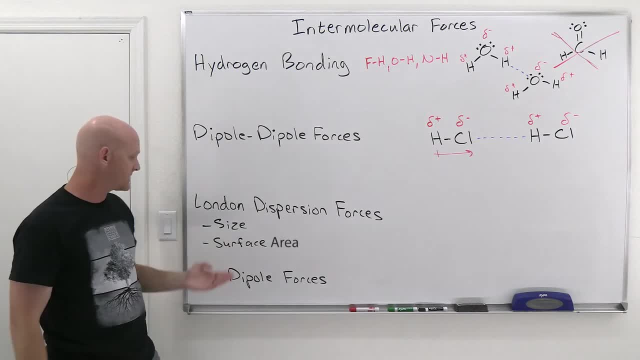 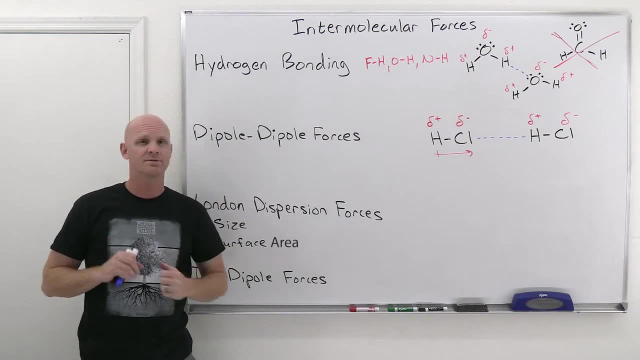 you have more surface over which these forces can interact between molecules, And so that plays a role as well. But size is probably going to be the chief one you compare in this class. So when you get to organic chemistry, if you get to organic chemistry, 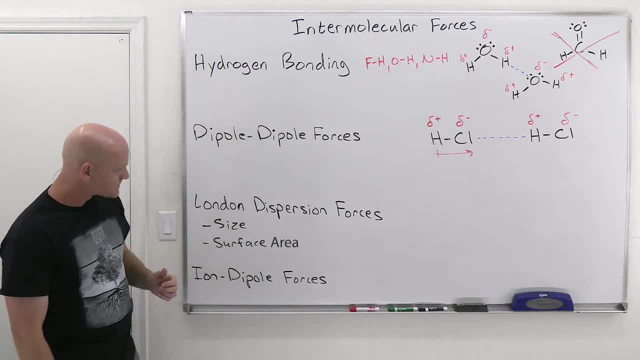 you're going to have to probably deal with this one a little more as well. All right, So all molecules have London dispersion forces, all of them. The question is, do they also have dipole-dipole forces or hydrogen bonding? So, but at the very base level, they're always going to have these. 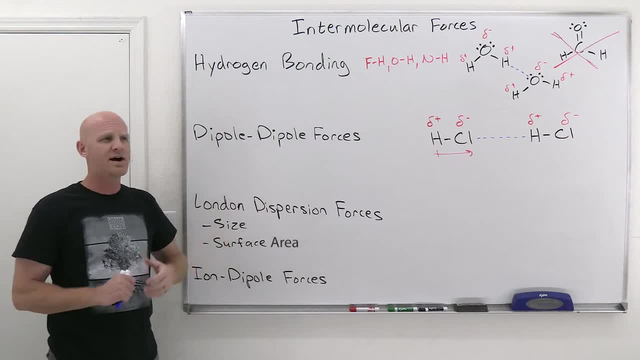 and the bigger the molecules, the more they have. Now, how are you going to figure out how big a molecule is? Well, usually, again, surface area does play a role And in certain questions I could totally, like you know, make sure that's something you need to know. 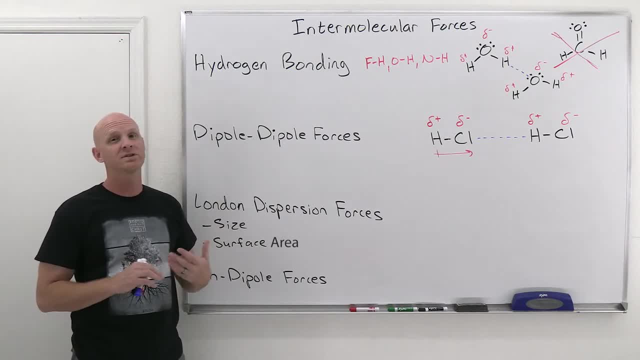 But more than likely, it's probably going to be just simply that's a function of molecular weight. So as long as you've got molecular weights that are within, say, 10 or 15 percent of each other, This probably is not going to be the deciding factor. 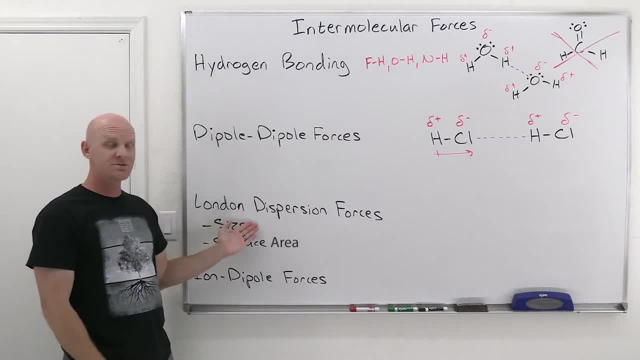 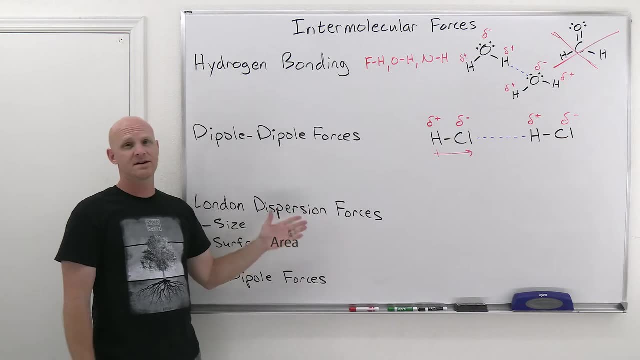 However, if you've got significant differences in molecular weight, London dispersion forces can end up being the deciding factor, And we'll see some examples of when that comes about. Cool, But the big thing is this: non-polar molecules. This is all they got. 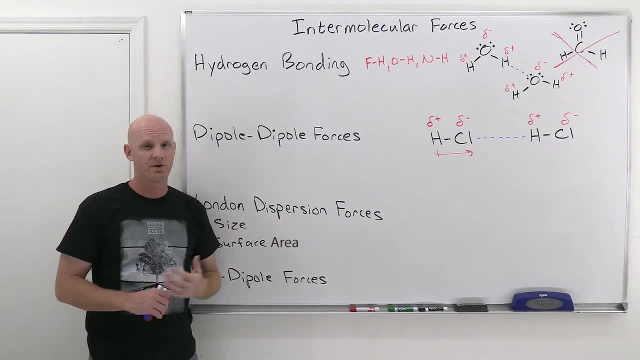 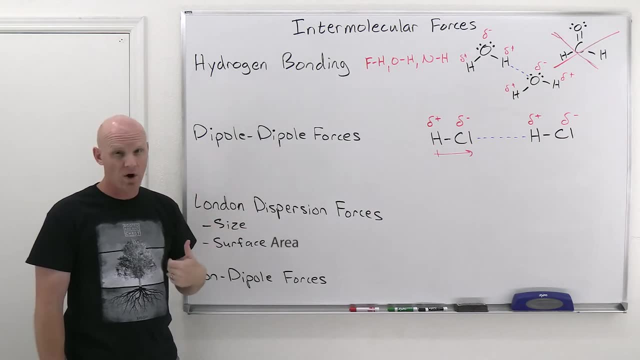 And so that this is going to be most relevant when we're talking about non-polar molecules, Whereas polar molecules, not only are they going to have London dispersion forces, they're also going to have dipole-dipole forces, And if those polar molecules have one of the three most polar bonds, 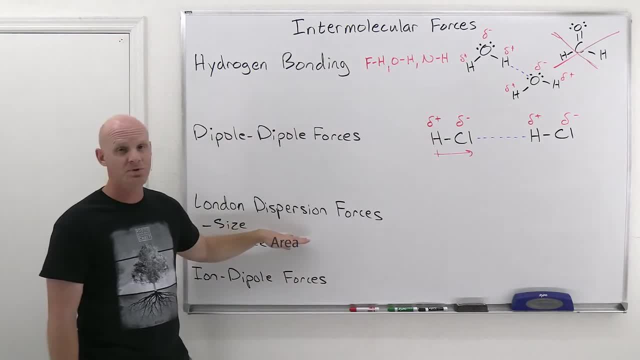 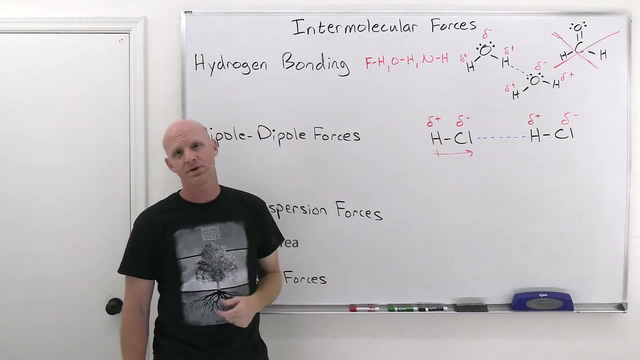 we're going to discuss this FH, OH or NH bond, then, in addition to the London dispersion and dipole-dipole, then they're also going to have hydrogen bonding and they'd have all three. So, like water, molecules could have all three of these intermolecular forces, it turns out. 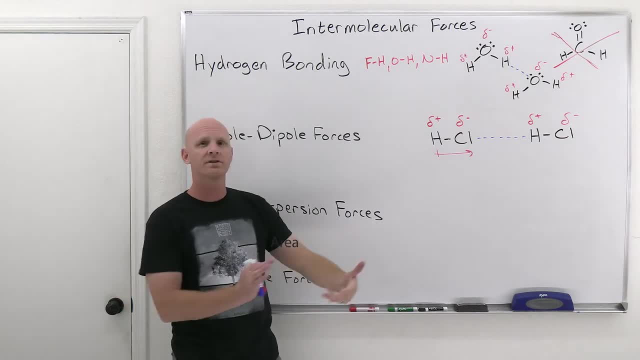 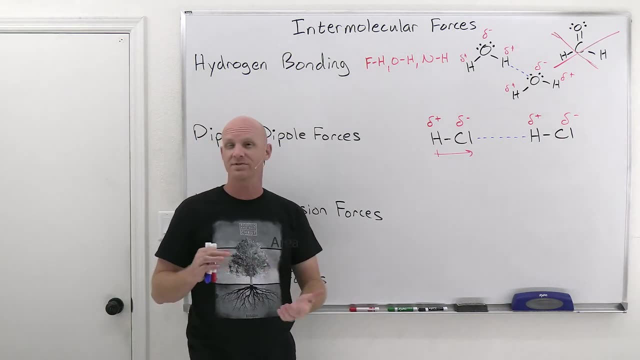 So sometimes you'll get questions that ask you: list all the intermolecular forces that are possible, So, but you know, just as common as probably list the strongest intermolecular force that exists for this molecule and stuff like that. And you're supposed to realize that the general ranking is going up this way. 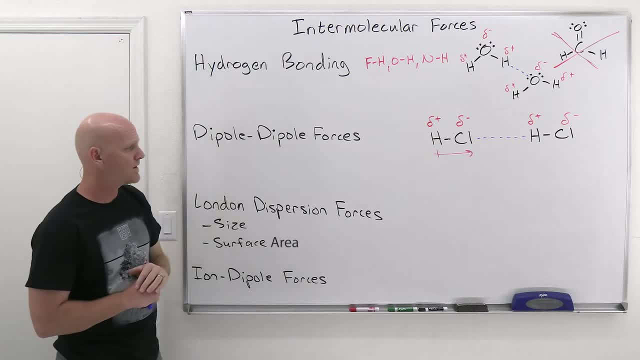 from London dispersion to dipole-dipole, to hydrogen bonding. Okay, Let's talk about ion-dipole forces for just a minute. So ion-dipole forces are actually quite commonly stronger than hydrogen bonding. So, however, we kind of discuss them separately from these three, because ion-dipole forces 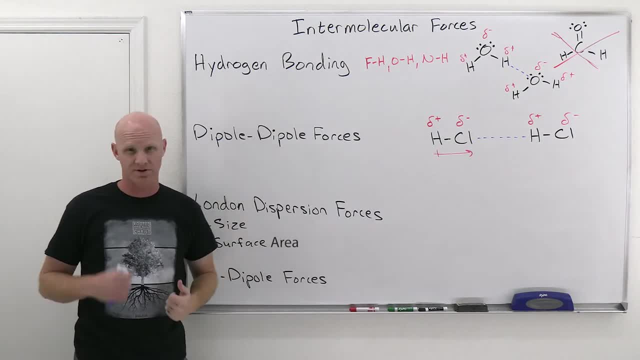 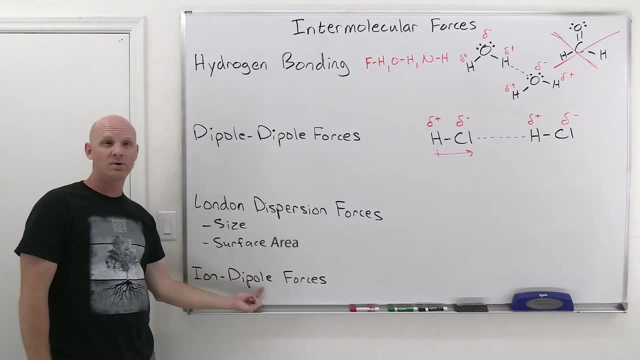 truth be told, I don't even think it's great to call them an intermolecular force. Again, intermolecular means between separate molecules. Well, ion-dipole forces are going to be between a molecule that's polar and has a dipole, and with an ion. 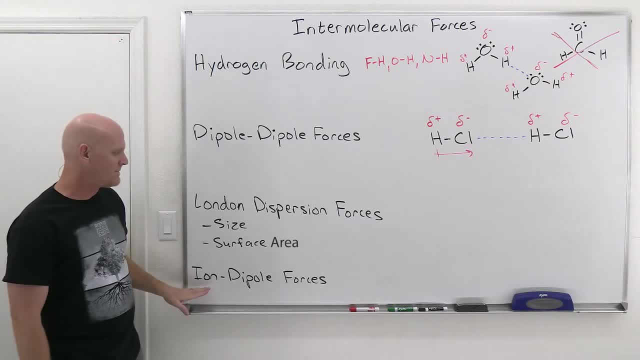 Well, ions aren't molecules, they're ions. they get a separate name And so, as a result, this really probably isn't, you know, properly classed in intermolecular force, even though it's grouped in here all the time and pretty much every textbook you're likely to see. 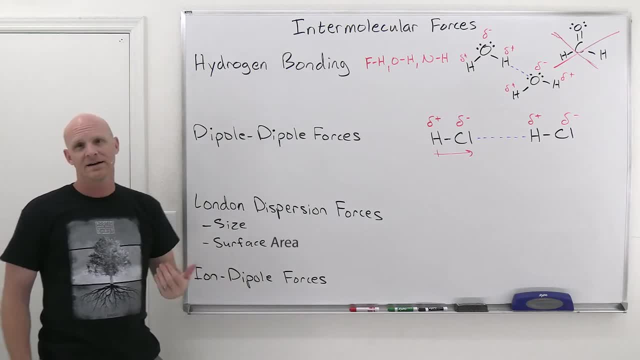 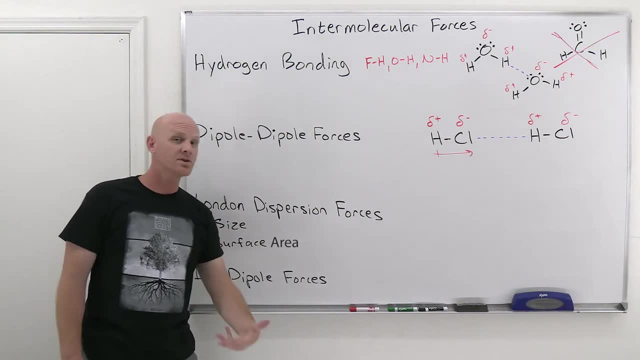 So, but this is going to be the force between a polar molecule and an ion, And so it automatically implies, therefore you have a mixture, And so we could never talk about ion-dipole forces in a pure substance and like a pure liquid. You've got to have a mixture, and the most common example you'll see is: you know, 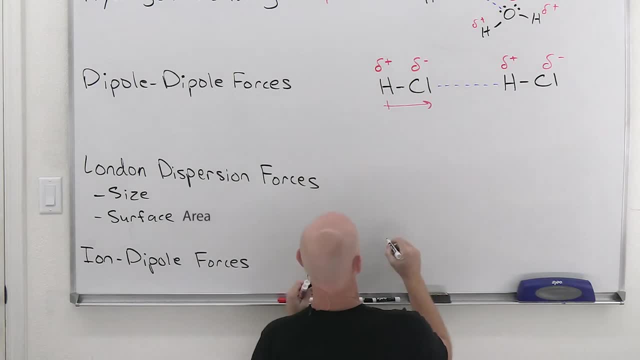 dissolve any ionic compound in water. So let's say, you know, I've got sodium chloride and I've got some sodium ions And I've got some chloride ions, And what you're going to find out is that the water molecules are going to surround the sodium. 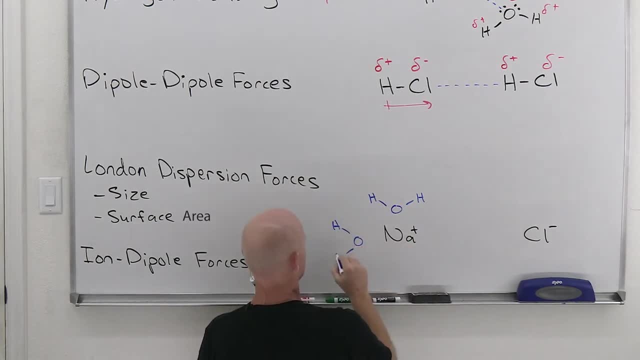 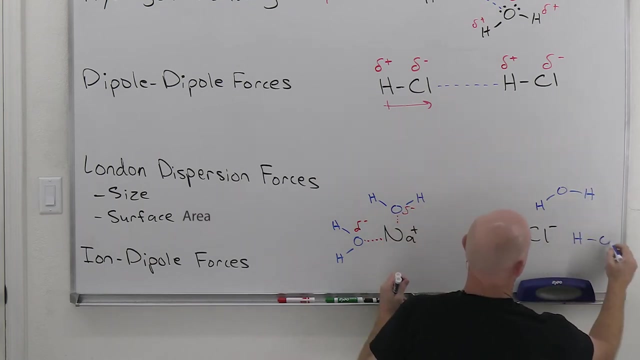 with the oxygens facing in, if you will. That way you get the partially negative oxygens interacting with the positively charged cations. Contrasting that over here with chloride, you're going to have the hydrogen atoms facing in, And so now you're going to have the partially positive hydrogens interacting with the anions. 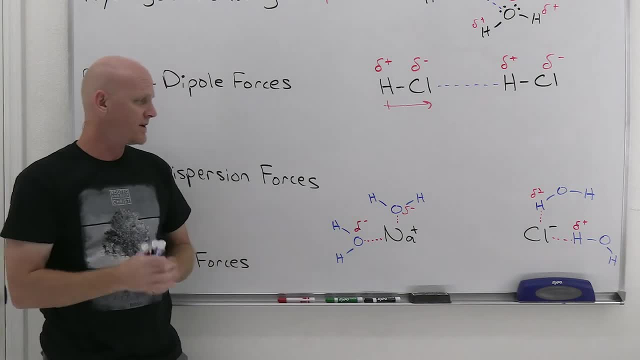 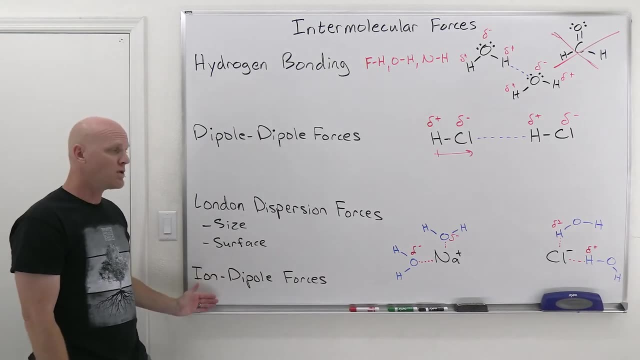 And I hear- I just drew a couple- there might be several of these different water molecules interacting with the cations and the anions respectively. So in the force of this interaction now we call- that's what we call- these ion-dipole forces, Cool- and it turns out there's a whole, you know, range of strengths here that are possible. 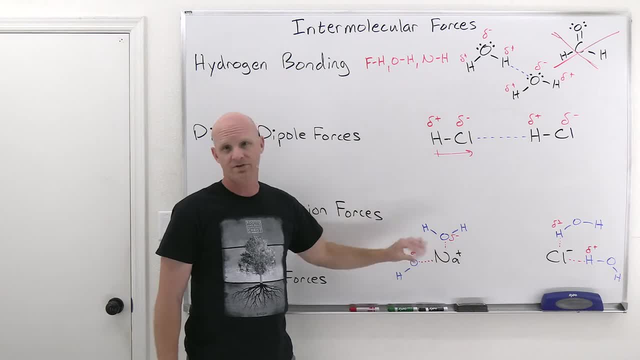 And it turns out that the smaller the ions, the greater the strength, and also it's going to be affected by charge. The more positively charged the cation, the more negatively charged the anion, the stronger these interactions as well. So it turns out that there's some overlap between the strength of these ion-dipole forces. 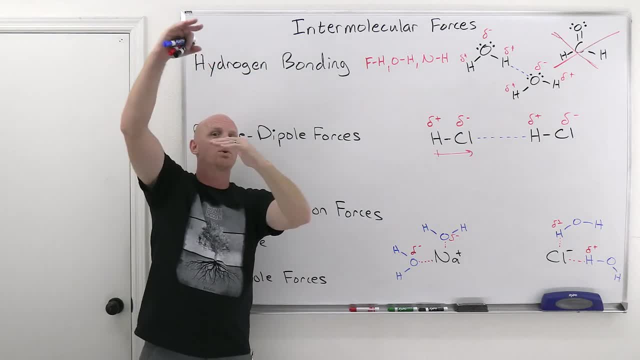 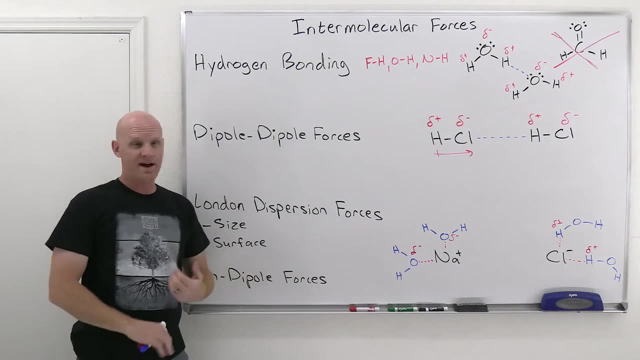 and the strength of the hydrogen bonding, But on average the ion-dipole force range is higher as a range overall than the hydrogen bonding range. Now, is every ion-dipole force stronger than every hydrogen bonding force? No, but again the overall range is higher, even though there's some overlap. 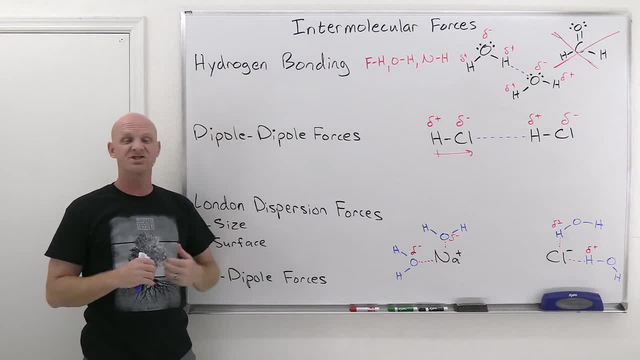 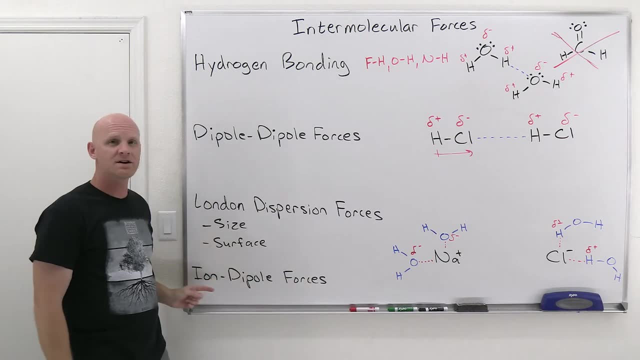 So keep that in mind. if you have to, you know, say which of these intermolecular forces you know in general is the strongest. you'd actually probably say ion-dipole. Cool, now for pure substances, though we rule this one out. It's not even a possibility for pure substances. 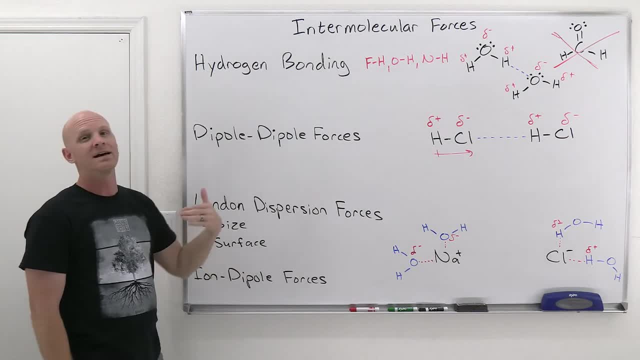 These would be the only three we'd actually consider, and so it wouldn't even be on the board. And so when you're looking at pure substances, hydrogen bonding is usually classified as being the strongest in that case. But we'll see some different comparisons you're likely to make and kind of. 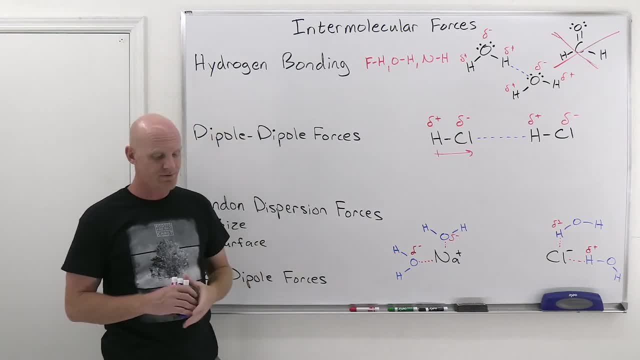 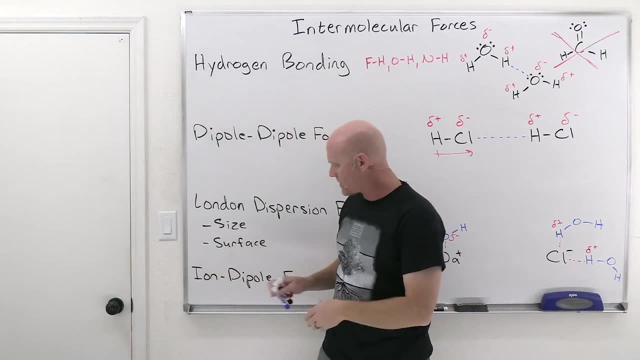 ranking these based on their overall strength, and we'll see one little surprise here. Okay, so it turns out these intermolecular forces affect some of the bulk properties in a liquid, And it turns out like the easiest one to kind of describe is boiling point. 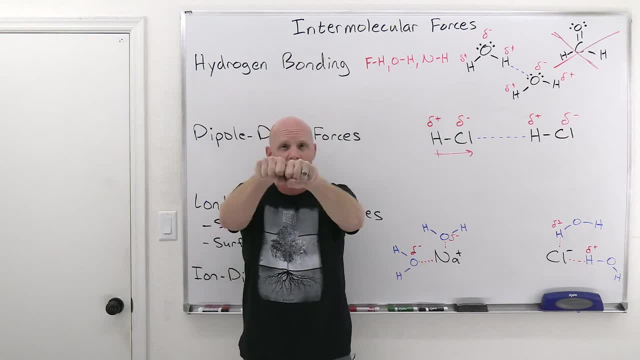 In boiling points you're going from a liquid to a gas. In the liquid phase, all the molecules are touching each other, Whereas in the gas phase they're spread out by large amounts of empty space. we learned in the last chapter, And so to go from where you're touching and in contact and experiencing these intermolecular forces. 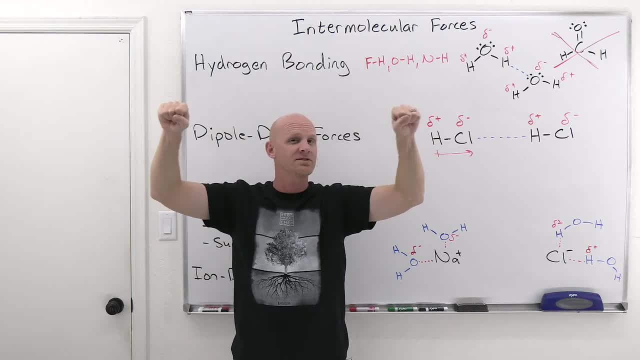 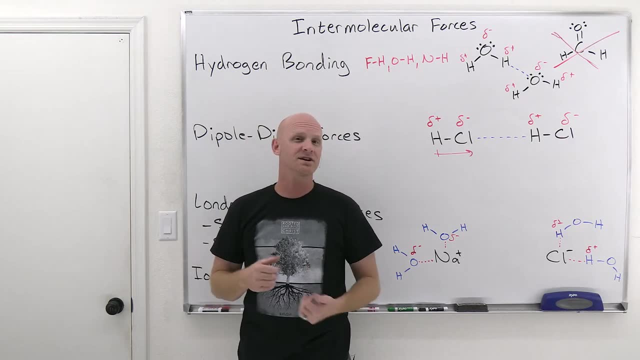 to where you're spread up by lots of empty space and not experiencing these intermolecular forces. So then, those intermolecular forces must be broken, And the stronger they are, the more energy it's going to take, And so you're going to end up with a higher boiling point. 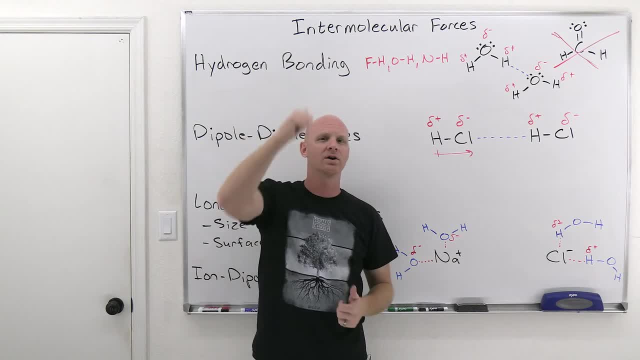 So greater intermolecular forces is going to lead to a higher boiling point. And so if I give you, you know, three compounds- we're going to do some sets here in a little bit- And I say which one has the overall highest intermolecular forces. 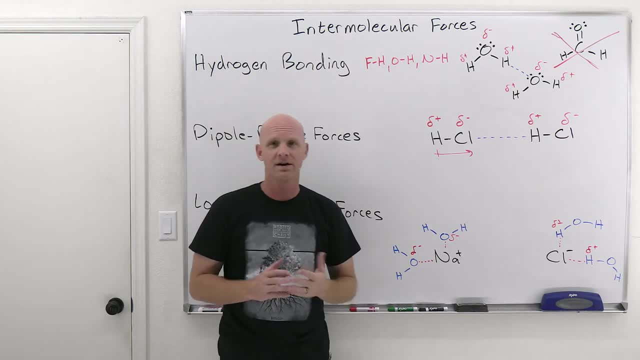 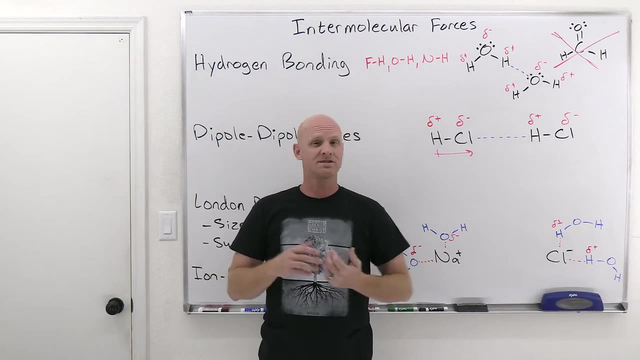 Well, we'll learn how we kind of make that comparison based on what we got available here, And the one with the greatest intermolecular forces. we'd also anticipate having the highest boiling point, But it turns out we probably anticipated having the highest melting point as well. 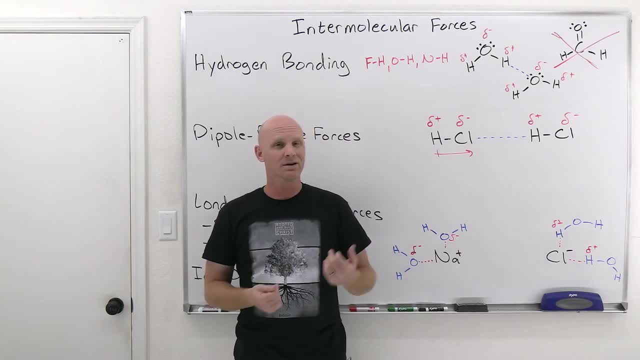 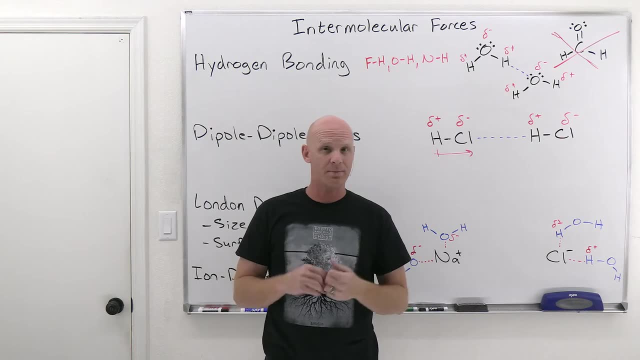 You've still got to break some of those intermolecular forces to go from solid to liquid. You're probably just going to break a whole lot more of them and going from liquid to gas- Cool. We also want to talk about the enthalpy of vaporization. 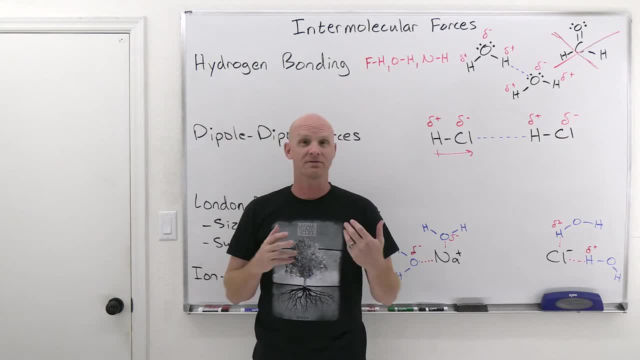 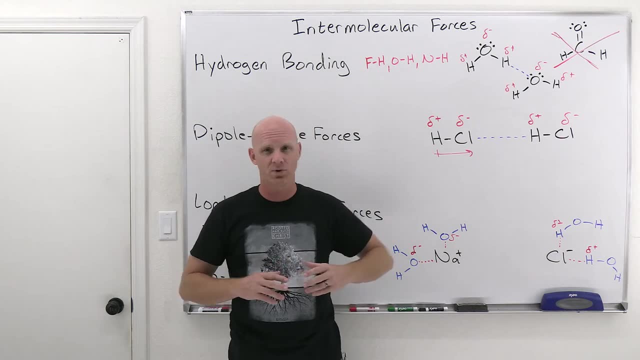 because we can talk about the temperature at which boiling happens, But we can also talk about the amount of heat at the boiling temperature that is going to be required to go from liquid to gas And that is also going to be higher for something with greater intermolecular forces. 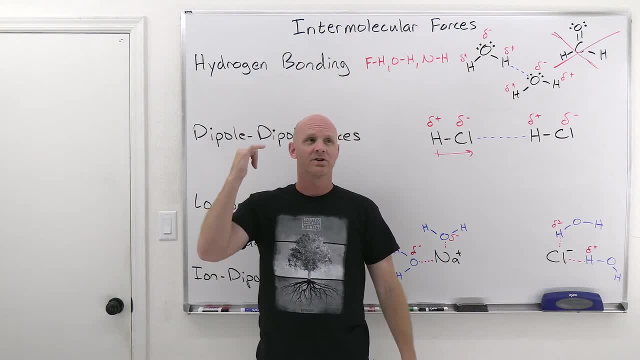 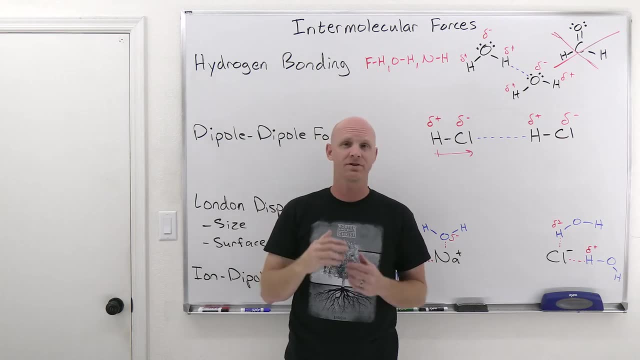 So right off the bat, we've seen that. you know, involving phase changes you're going to have with the greater intermolecular forces, you're going to have a higher melting point, boiling point, and your enthalpy of vaporization And technically, your enthalpy of fusion, which is melting, would also be higher. 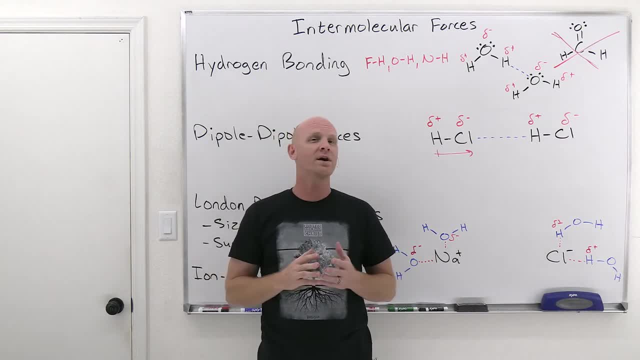 So all those associated with phase change is going to be higher. You're also going to have a greater what's called viscosity, So, and you kind of have an intuitive idea, probably, what viscosity means. And so if you pour a liquid, something that pours more slowly or more thickly is considered more viscous. 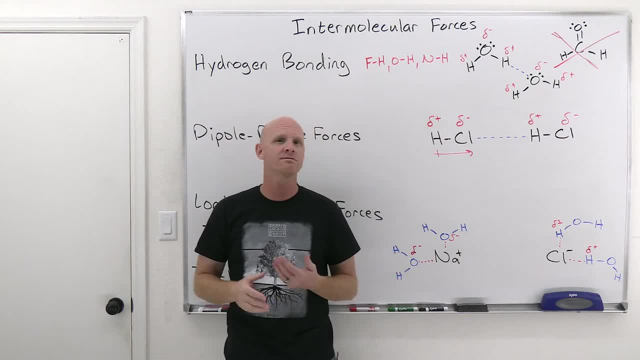 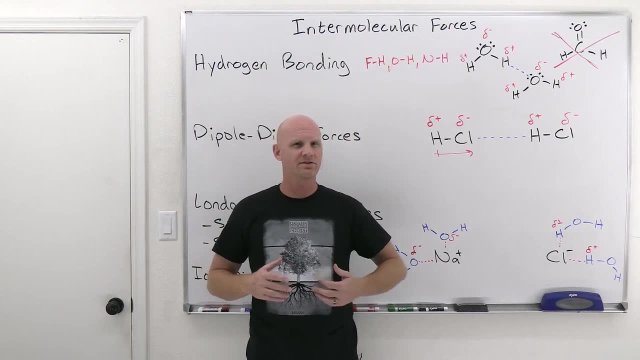 So like if you pour water and you pour honey, the honey is much more viscous, or motor oil, or something like this And the idea. you know, if you look at the technical definition of viscosity it doesn't seem to kind of jive with that. 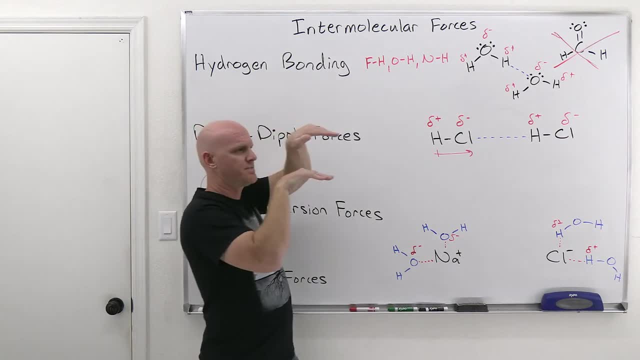 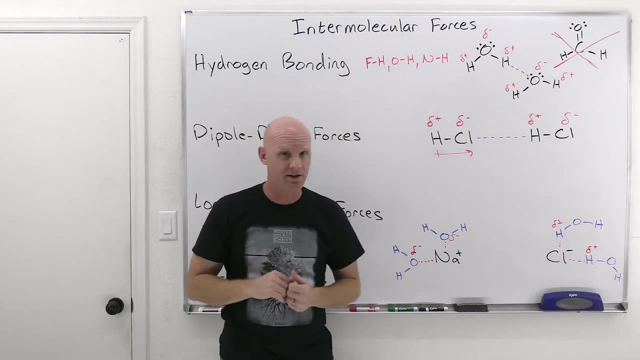 But you know, when fluids flow, they flow in layers, So, and when you have friction between the different layers of fluid flow, then they all want to flow together and flow more thickly, And the nature of that friction is intermolecular forces. 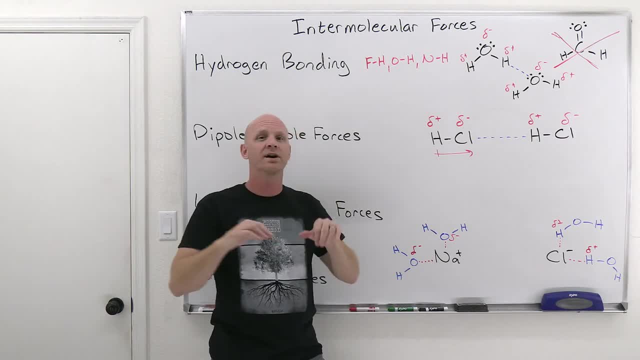 And so the greater the intermolecular forces, the greater the friction between the layers, and the more they're going to all want to flow together and flow more thickly, which is really what viscosity comes down to, And so there's something that you'd recognize by sight anyways. 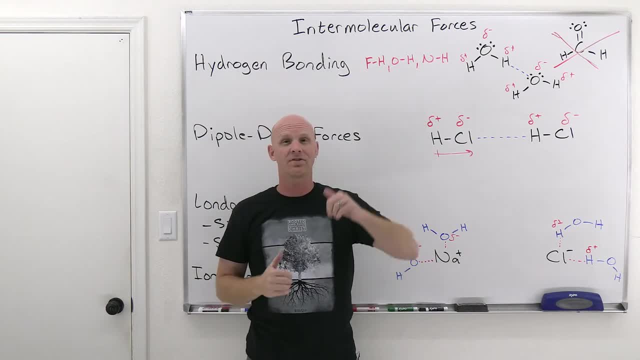 And so overall highest intermolecular forces is also going to lead to the highest viscosity as well. So it's also going to lead to the highest surface tension. So in surface tension, if you look at it is the you know when you're at the surface of a liquid. 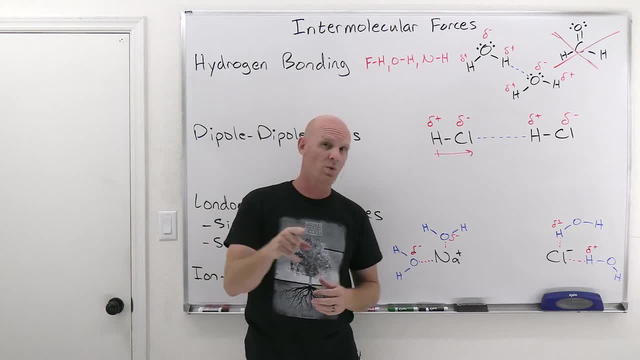 So you know, if I told you I had a friend and my friend can walk on water, So you might look at me a little funny and be like he's got friends with Jesus or something like this, And that would be true. 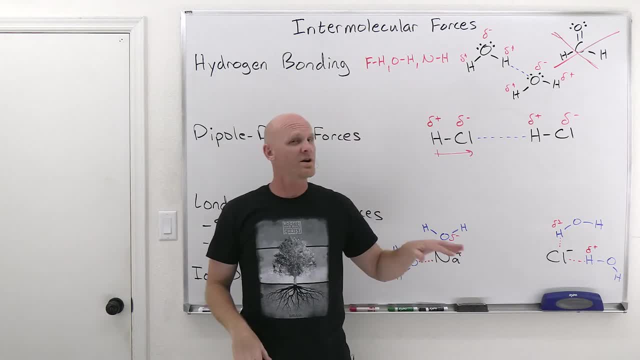 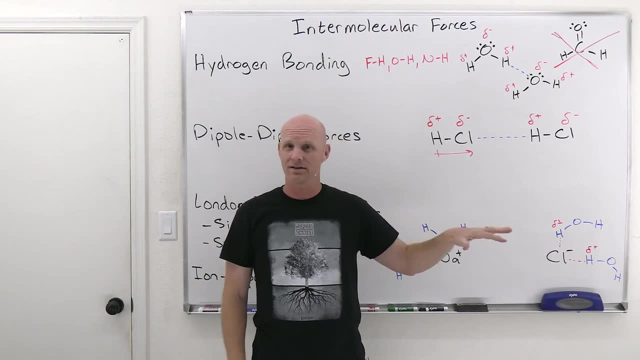 But you might also realize that I'm talking about a water bug And my friend the water bug, because I'm pretty lonely in this room filming all the time. So my friend the water bug can walk on water whereas I can't, but he can. 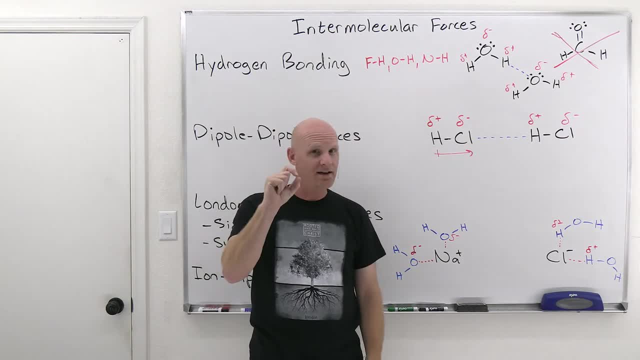 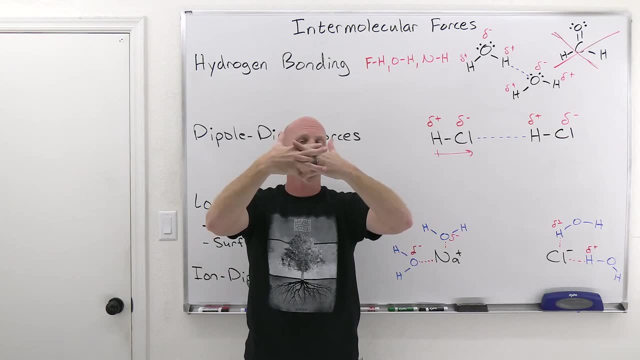 And the water bug can walk on water because he can spread his really tiny weight over a large surface area and not puncture this network of hydrogen bonding on the surface of water. And that hydrogen bonding network at the surface is what provides that surface tension. 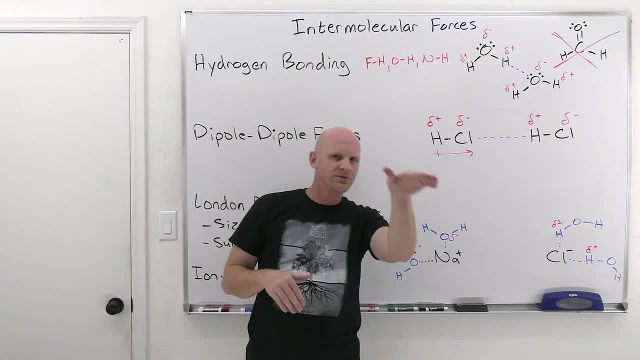 So it's why you can fill up a glass of water a little fuller than the actual top of the glass If you try. you know, if you add water drop by drop, slowly it'll actually bubble up at the top And that's also a function of that surface tension. 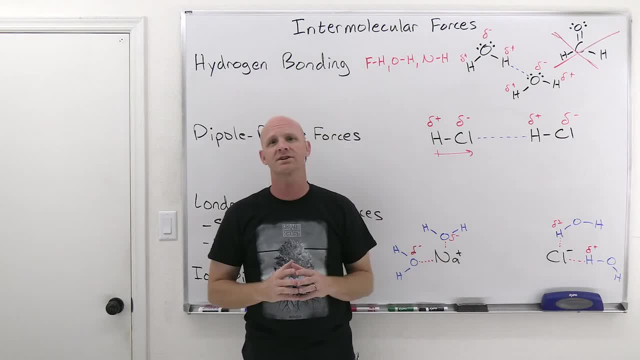 And so it turns out, the greater the intermolecular forces, the greater the surface tension, on a liquid as well We'll talk about. higher intermolecular forces will also lead to a higher critical pressure and temperature, which I'm going to reserve talking about. 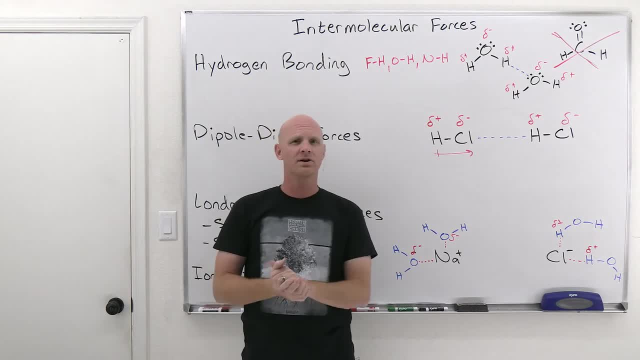 in the next lesson when we talk about phase diagrams. But the one thing that's going to go lower: if you have a higher intermolecular forces, you're going to end up with a lower vapor pressure. We'll talk a little more about vapor pressure in a minute. 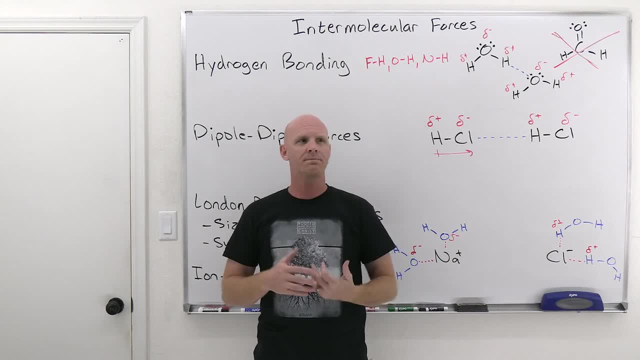 But vapor pressure really is a measure of how much. you know what fraction of the molecules in a liquid have actually jumped out of the liquid into the vapor phase, And it turns out for that to be possible they have to have a ton of kinetic energy. 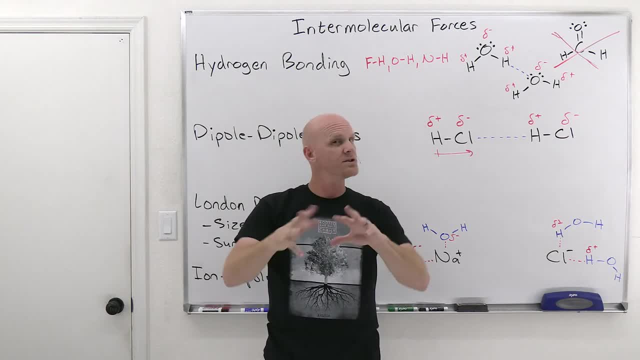 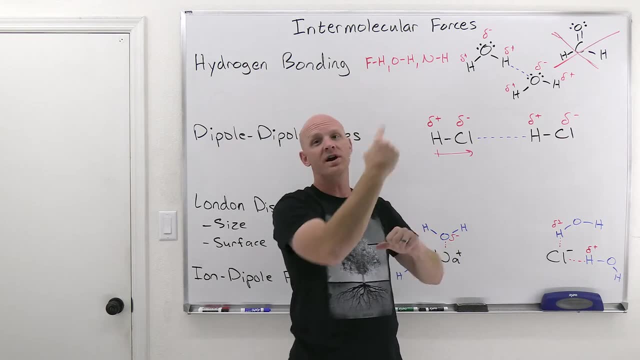 enough kinetic energy to jump out of the liquid, even though all the liquid molecules are, you know, in contact and touching each other and attracting each other. So you have to have enough kinetic energy to overcome that jump out. Well, you know, the greater that you know. 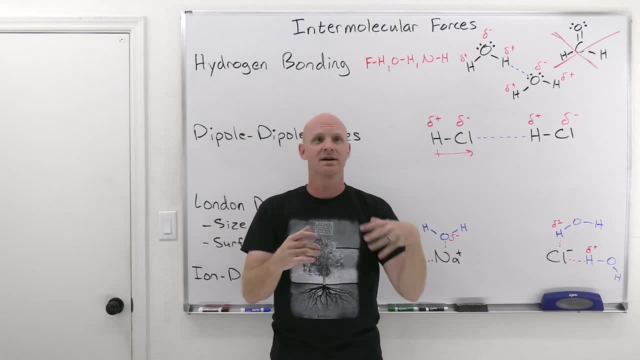 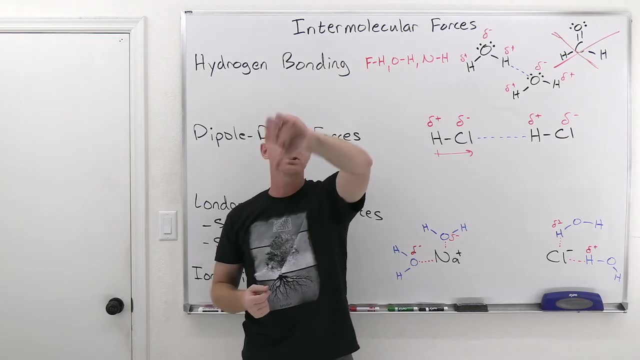 that stickiness of the molecules, that intermolecular forces in the liquid phase. So then the smaller the fraction of molecules that would actually have enough kinetic energy to jump out. You might recall that you know there's a distribution of kinetic energies. 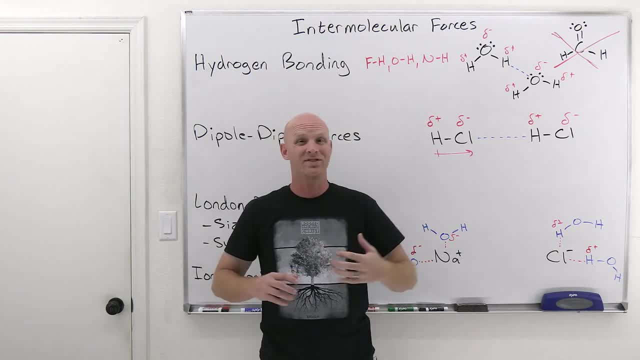 and molecules. that we learned in gases. it's true in liquids as well. So, and the stickier the molecules are, the you know, the fewer the percentage of molecules that would have enough to get out And you'd have a lower vapor pressure. fewer molecules in the vapor phase above that liquid. 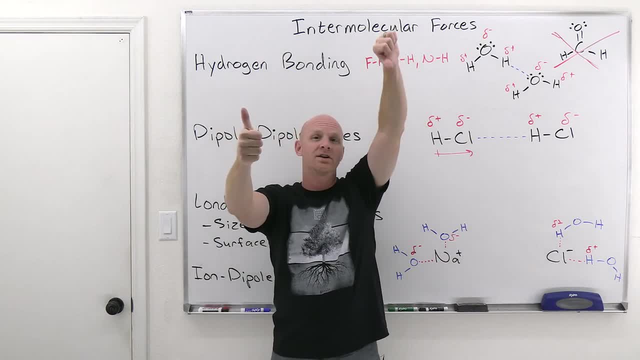 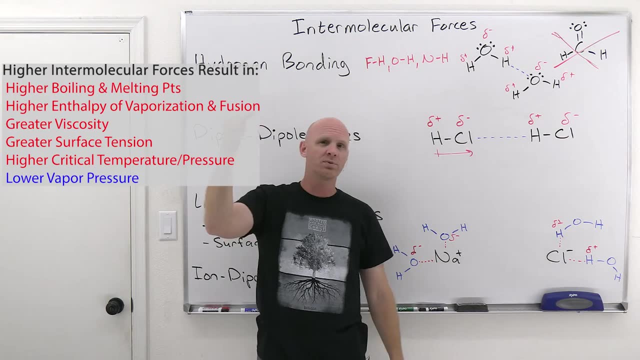 So a higher intermolecular force in a compound is going to actually lead to a lower vapor pressure, And so that's the one. that's kind of contrary. So higher intermolecular forces leads to higher boiling points and melting points, enthalpies of vaporization and fusion, higher viscosity, higher surface tension. 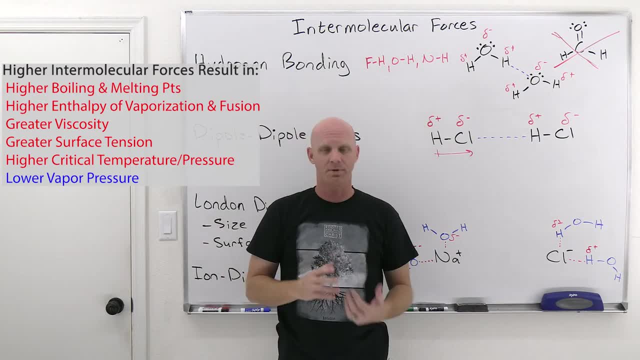 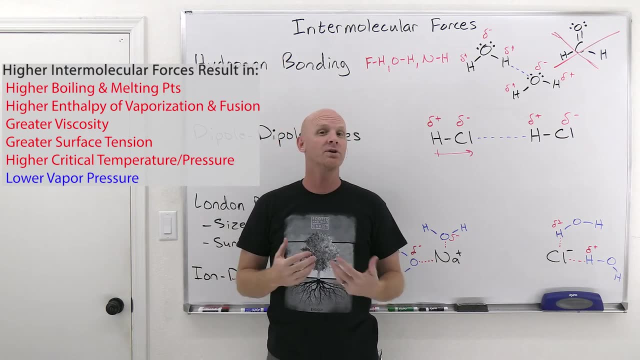 higher critical temperature and pressure but a lower vapor pressure. So we're going to rank some compounds here in a little bit and we're going to rank them based on having the highest overall intermolecular forces And the ones with the highest overall intermolecular force. 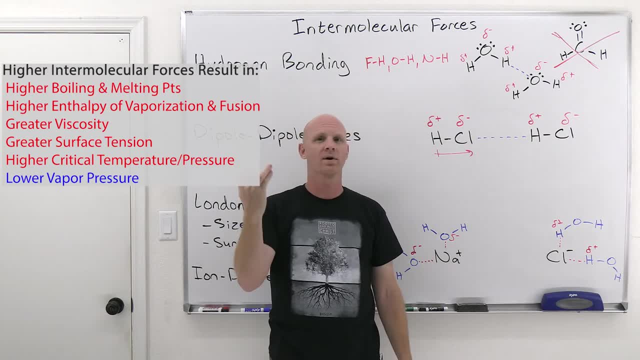 forces would also have the highest boiling point, highest melting point, highest enthalpy of vaporization, highest enthalpy of fusion, highest surface tension, highest viscosity, highest critical temperature and pressure, but the lowest vapor pressure. And so, instead of asking you a question just based on overall greatest intermolecular forces, 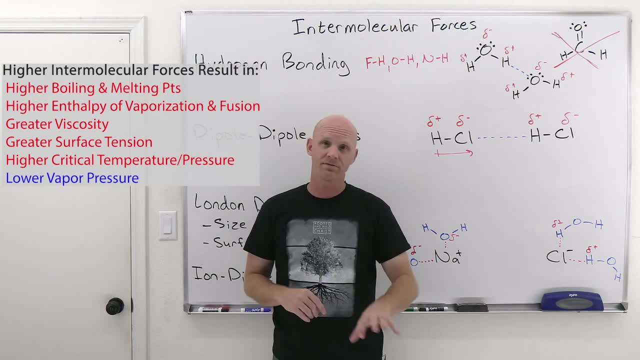 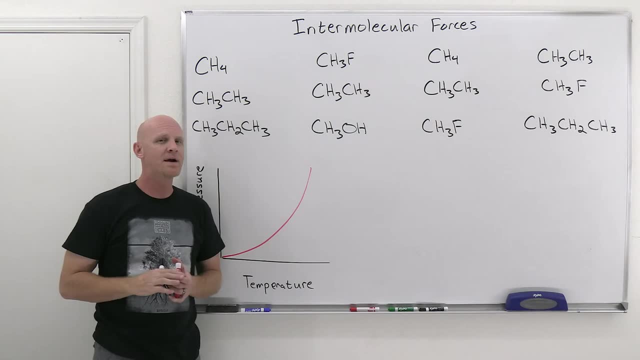 you could be asked one for greatest or lowest on any of these bulk properties of a fluid as well, And you should know how that functions. All right, let's take a look at some examples here. So before we compare intermolecular forces, 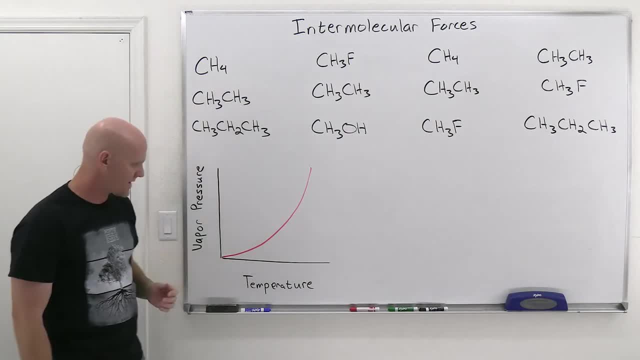 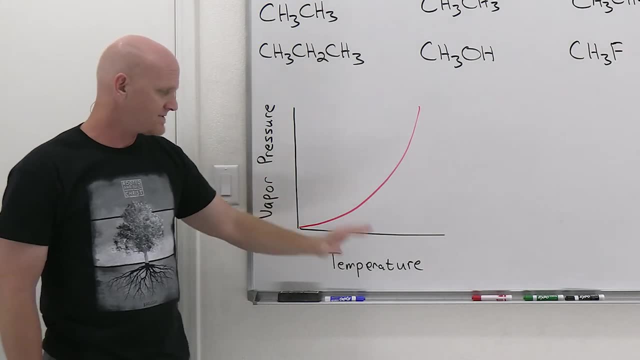 and some different sets. I did want to mention one more thing about vapor pressure. And if we look at what's called a vapor pressure curve here and we're going to have vapor pressure plotted on the y-axis here in Tor and temperature in Celsius on the x-axis, 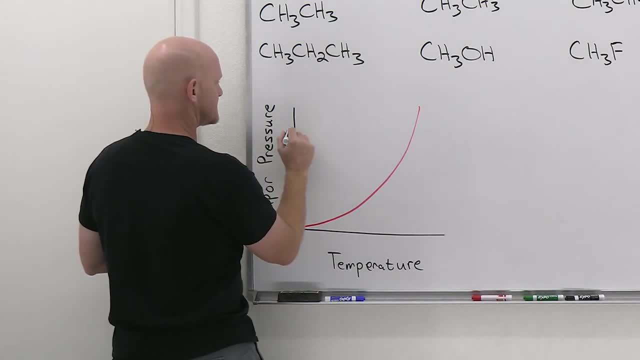 And it turns out. one thing you're definitely supposed to know from something like this, and something you're supposed to take away, is boiling point- What boiling point actually is. And we know it's the phase change between liquid and gas, But it turns out it's often defined and actually most probably defined. 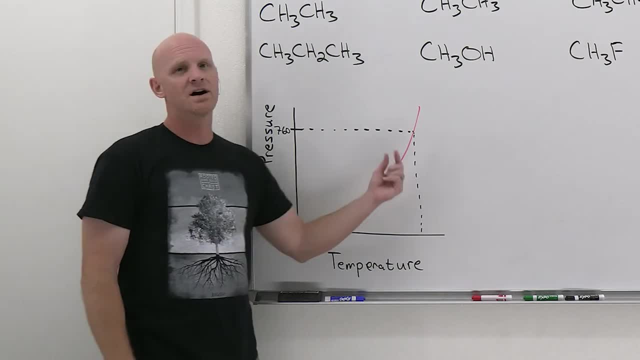 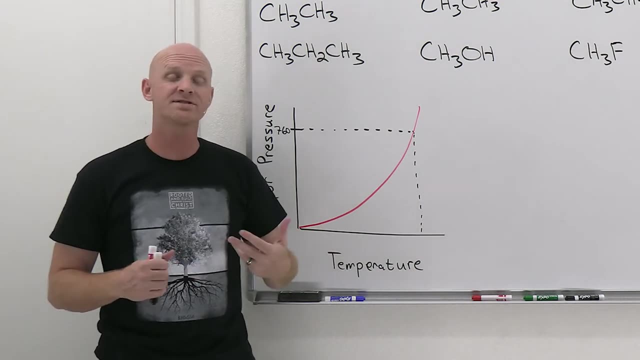 in terms of vapor pressure. So it turns out, as you heat a substance up, you're going to get more and more vapor because you're going to be giving more average kinetic energy to the molecules in the liquid phase, and so a greater percentage will have enough to get up into the vapor phase. and life is good. 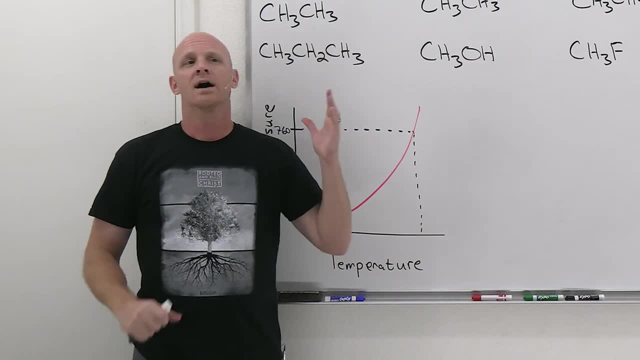 And this is something you intuitively know. If you said, you know, if I asked you: hey, I'm going to put one of two things in front of you. I'm going to put a turd on a plate in front of you. 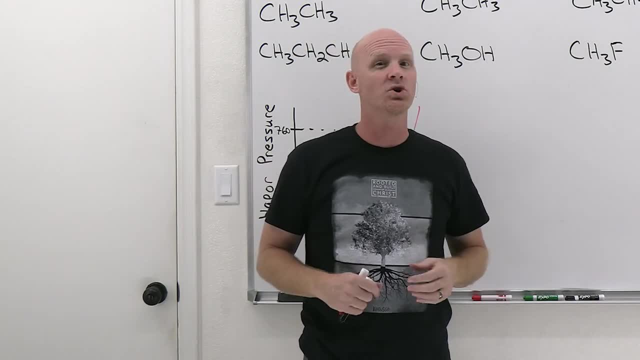 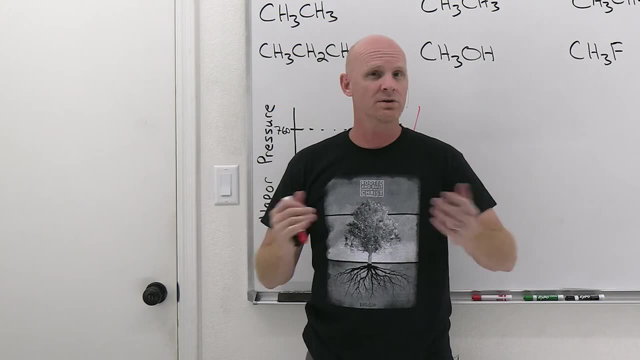 One is coming out of the oven and one is coming out of the freezer. Which one do you want? And when I asked students this in person, they almost always say the one out of the freezer, And you would intuitively know this right. 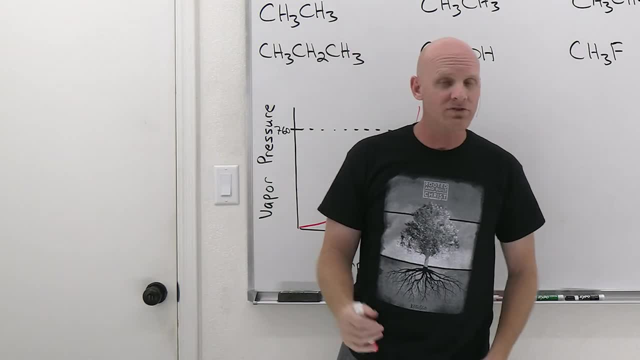 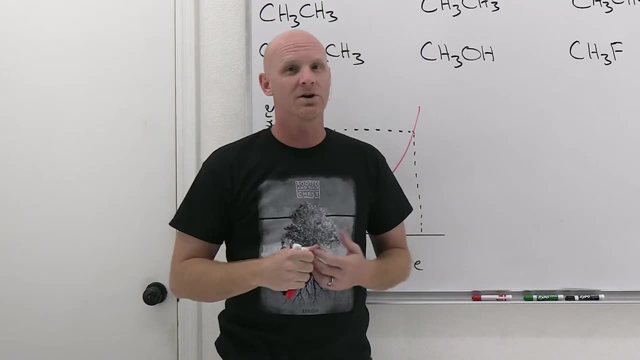 Because you like them crunchy. No, because it's going to smell less coming out of the freezer. Same thing. So solids have a vapor pressure associated with them too, And the hotter something is, the more vapor it's, you know. 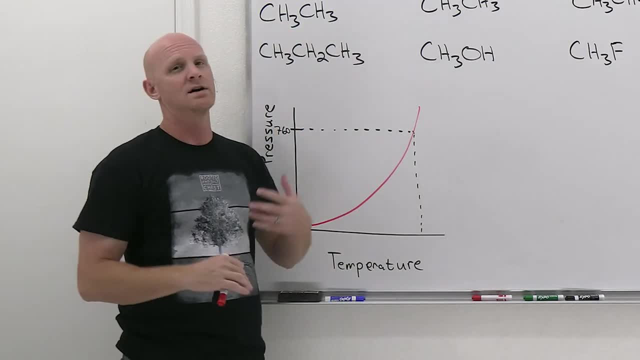 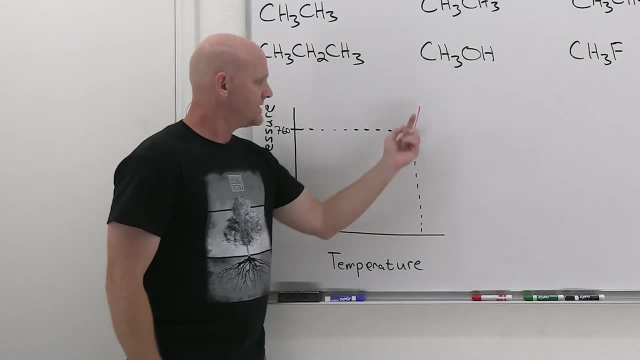 it's going to be giving off the higher its vapor pressure. So intuitively, you know this: As you heat something up, it's going to have a higher vapor pressure. So it turns out. it's not linear typically, So it's going to have this lovely logarithmic kind of curve here. 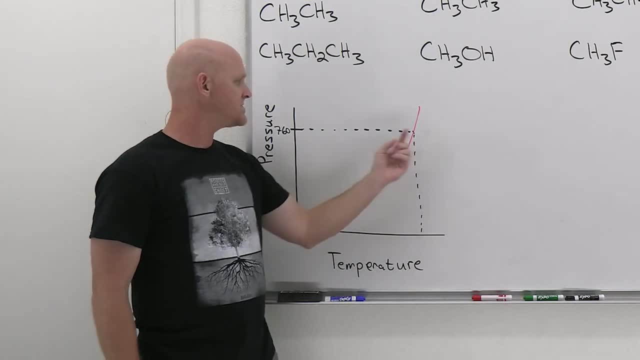 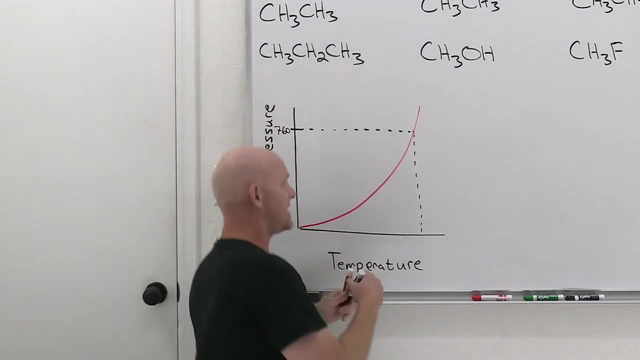 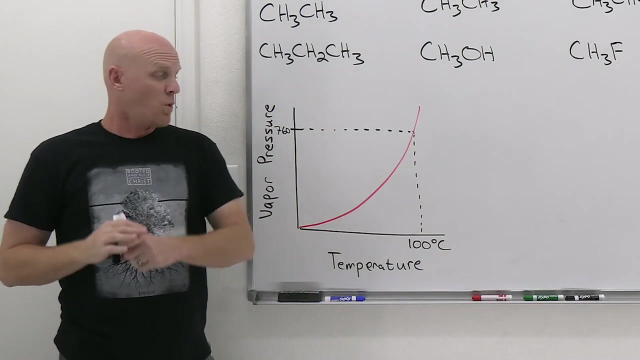 And if you look at water, when water's vapor pressure reaches 760 torr, ie 1 atmosphere, that's when it boils at sea level. And so it turns out that temperature, you know quite well, corresponds to 100 degrees Celsius in the case of water. 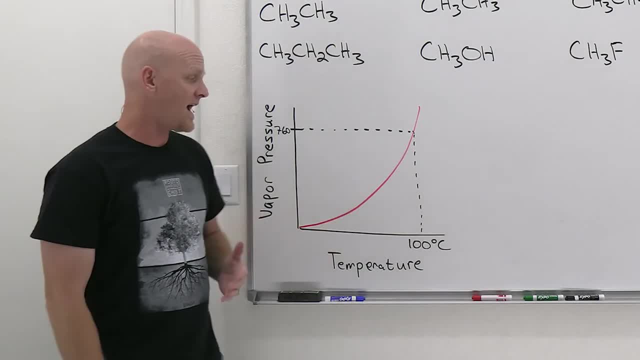 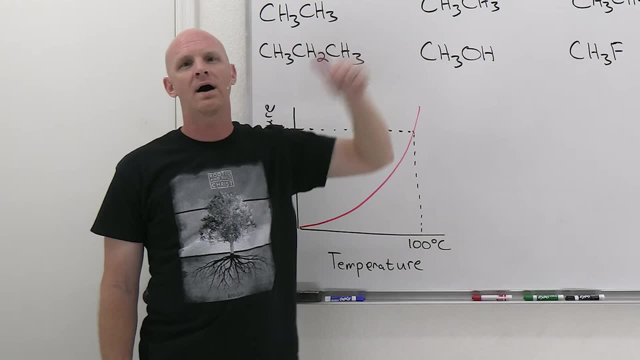 And so you know, if you want to boil water, that's what has to happen. The vapor pressure has to equal its external pressure. Well, if you go, you know, climb up to the top of a mountain, you're no longer actually going to be. 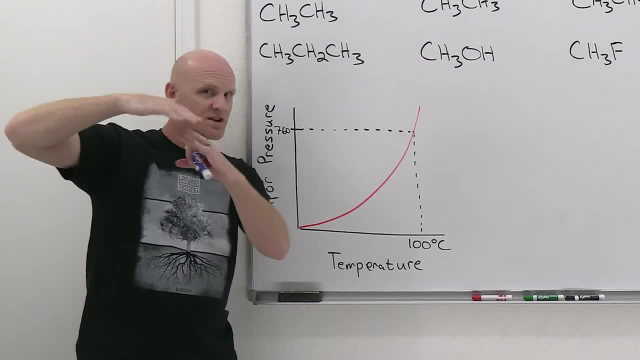 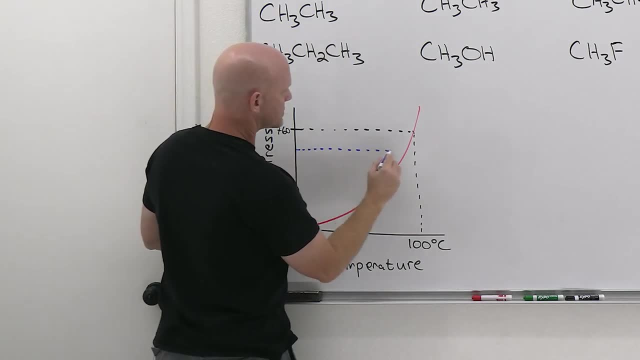 at 1 atmosphere, at 760 torr, you're going to be at some lower pressure because there's not as much atmosphere above you weighing down on you anymore. And so you know, let's say you just go to some lower atmospheric pressure. All of a sudden. now, the temperature you have to get to, so to where your vapor pressure is going to reach that atmospheric pressure, is not going to be 100 degrees Celsius anymore, It's going to be lower. And so you know, at the top of some tall mountain it might only be 90 degrees Celsius. 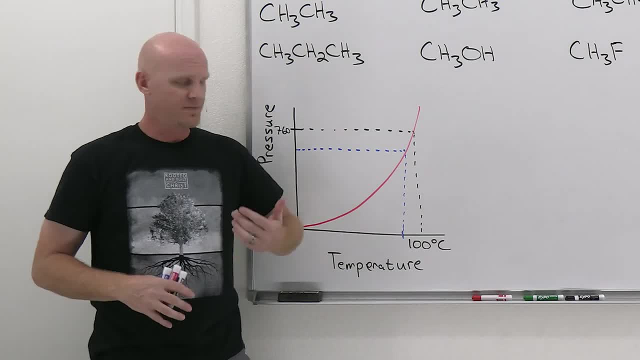 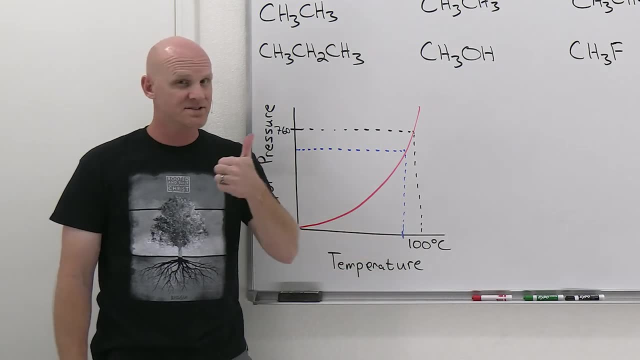 And so this is a problem. if you're cooking food, If you know, normally it says, hey, cook your rice for 10 minutes, So and boil it for 10 minutes. Well, if you're boiling at 100 degrees Celsius, that's great. 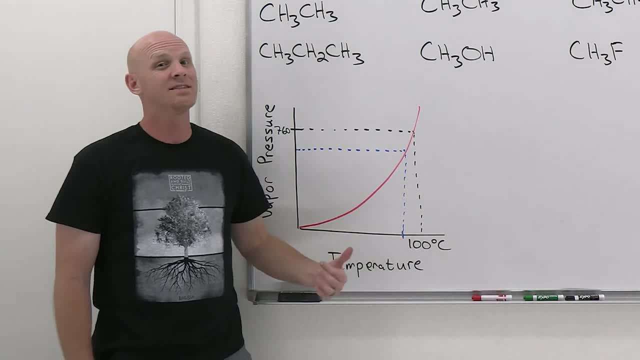 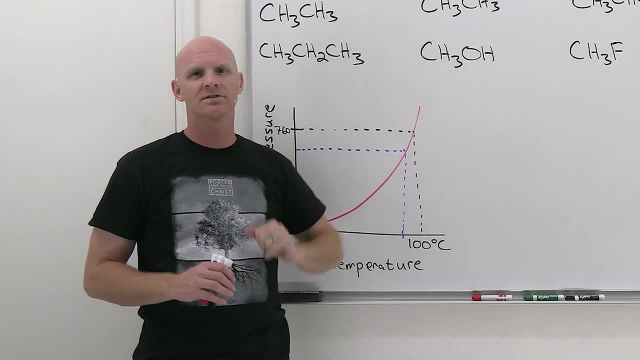 But if you're only boiling it at 90 degrees Celsius because you're on the top of a tall mountain, then you're going to have to actually cook it longer at this lower temperature, And so there's all sorts of special cookbooks for high elevation cooking and stuff like this. 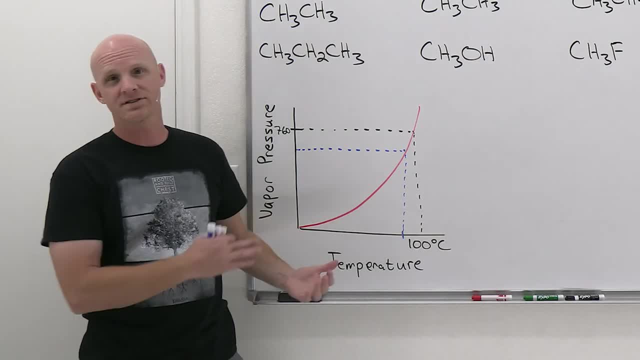 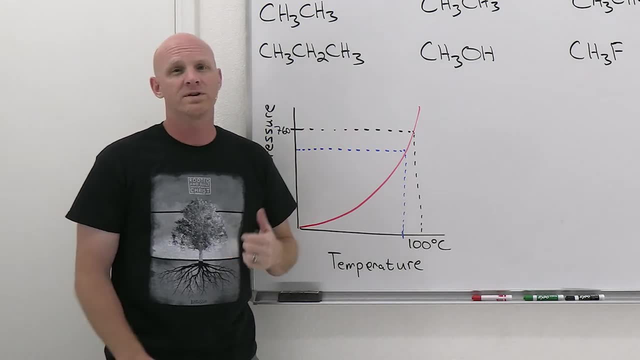 because things just don't cook the way they do at lower elevations for this kind of reason and stuff like that. So cool. So that's all I want to mention about vapor pressure. but you should realize again that when your vapor pressure reaches your external pressure, 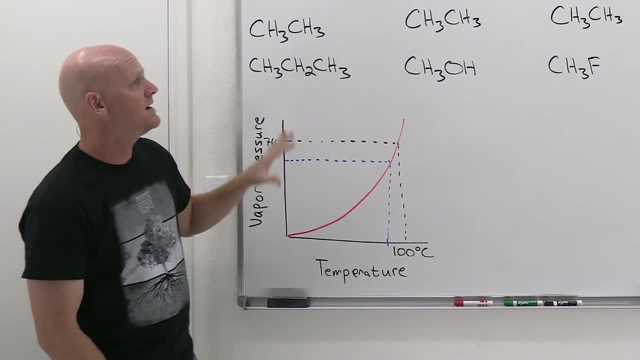 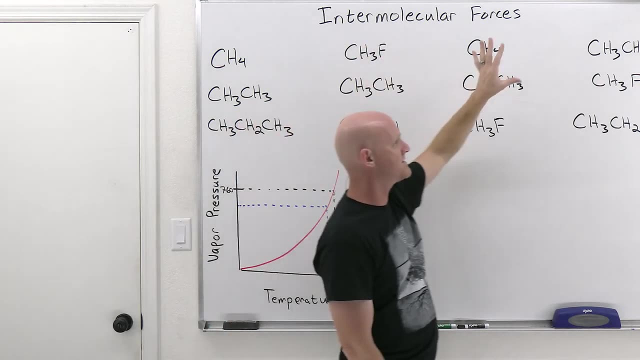 that's when a substance boils All right. So now we're going to do four different comparisons here. We're going to look for the highest intermolecular forces present in any one of these sets of three compounds. And first thing we should realize is we're just looking for what types of intermolecular forces are present. 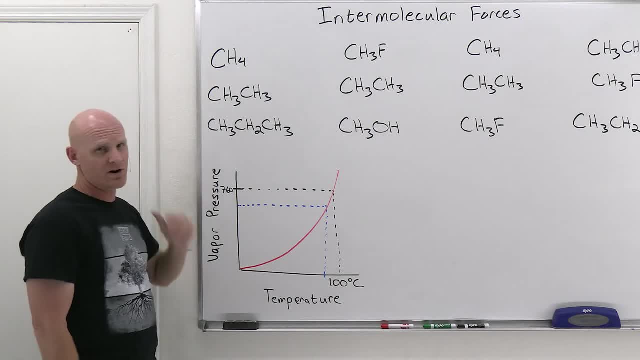 And so, if we start with this first set, all of these are hydrocarbons. They only have carbon and hydrogen, And so molecules with only carbon and hydrogen, well, those are nonpolar bonds, And if all your bonds are nonpolar, then you're going to be a nonpolar molecule. 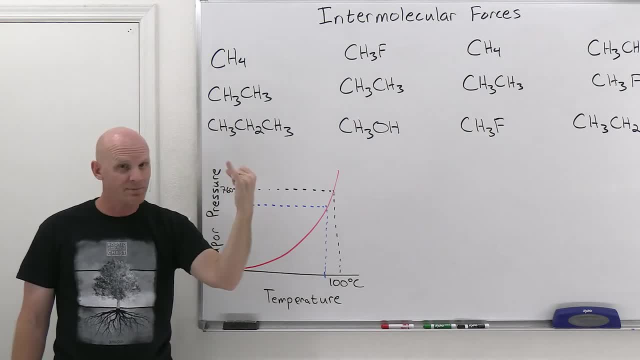 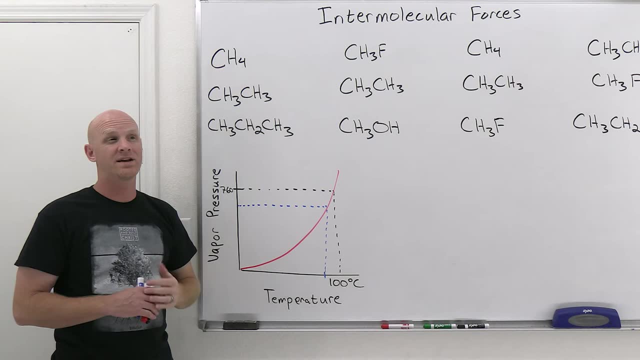 And so if all these are nonpolar molecules, well then they definitely don't have hydrogen bonding and they don't have dipole-dipole forces either, So they only have London dispersion forces. And if you're comparing molecules that only have London dispersion forces, 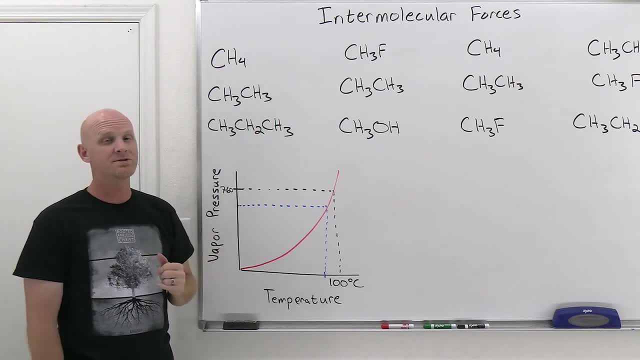 well then it comes down to size and surface area, And most of the time in general chemistry it'll be size. In organic chemistry you'll see some surface area kind of questions more commonly, But most of the time in gen chem it'll be about size. 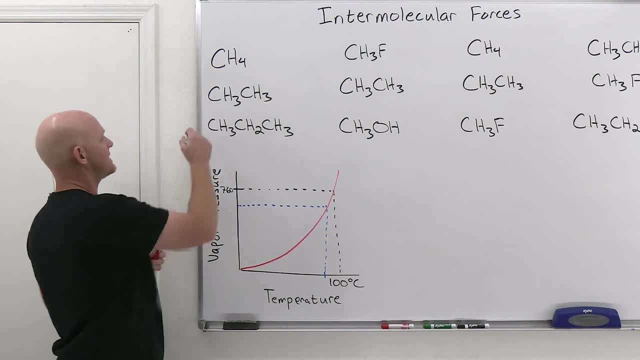 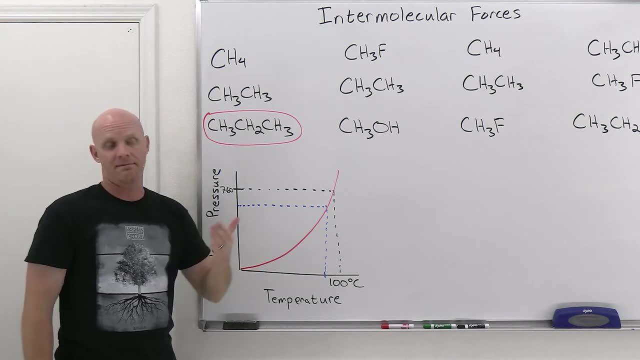 And if you look at these, it's easy to see who's the largest in size and that is going to be the one that has the overall greatest intermolecular forces out of these first three. Now again, my question is: who's got the greatest intermolecular forces? 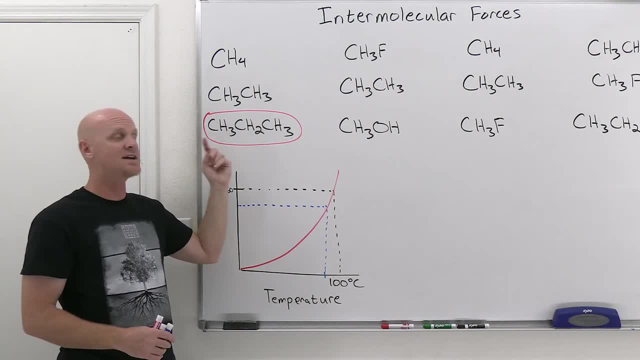 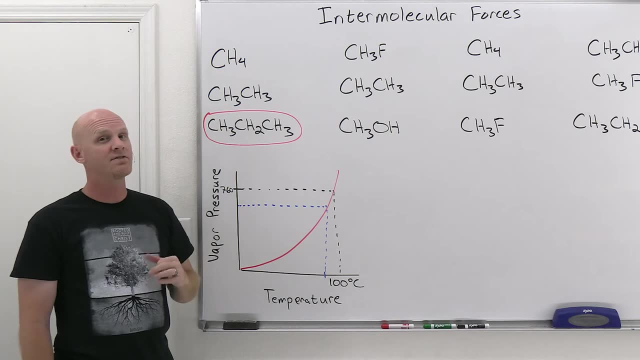 But notice, you would have given the same answer if I said who's got the highest boiling point, highest enthalpy of vaporization, highest surface tension, highest viscosity, But if I said who's got the highest vapor pressure, you wouldn't choose him. 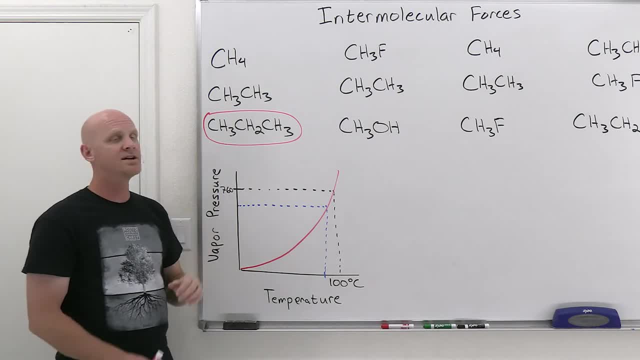 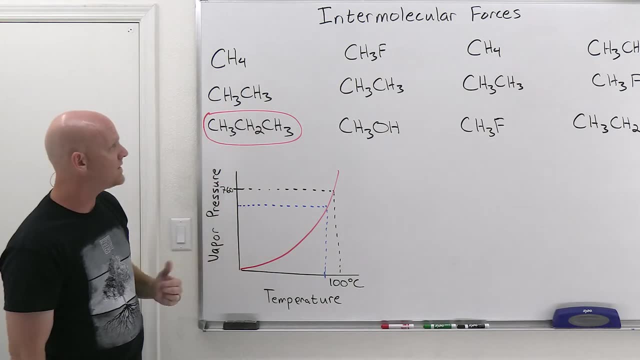 He's got the lowest vapor pressure. So just realize, once you can identify who's got the highest intermolecular forces, he's going to have the highest whole slew of things but the lowest vapor pressure. Cool, If I said who's got the highest vapor pressure. 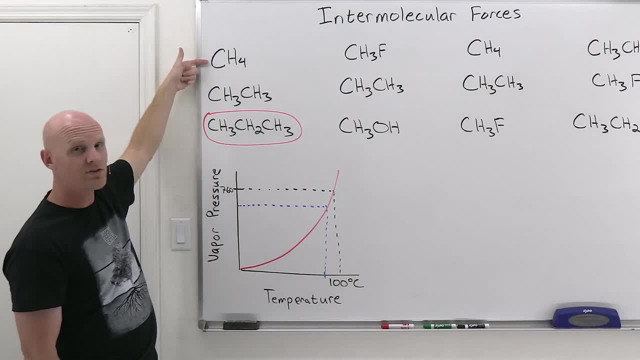 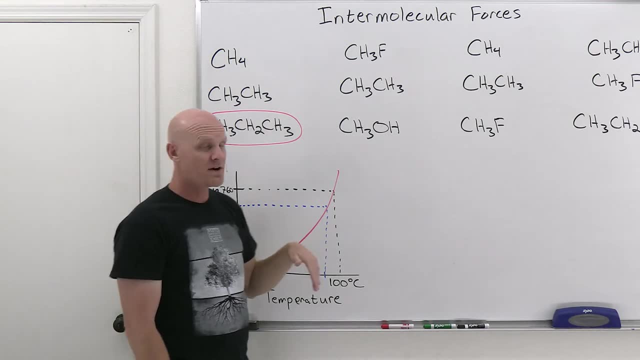 well then, you'd actually go the other direction and pick the one that has the lowest overall intermolecular forces, in this case CH4.. OK, so that's one comparison you might be called to make. The next comparison you might be called to make is when your molecules are all. 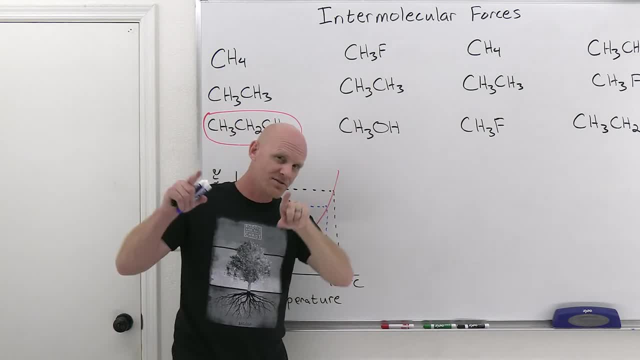 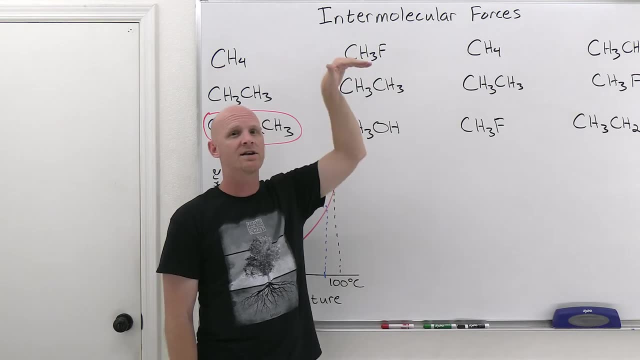 very similar in size. and when they're very similar in size, that is when it's most appropriate to talk about London dispersion forces being weaker than dipole-dipole forces and dipole-dipole forces being weaker than hydrogen bonding. And so if we compare these three, so the middle one here, CH3CH3,. 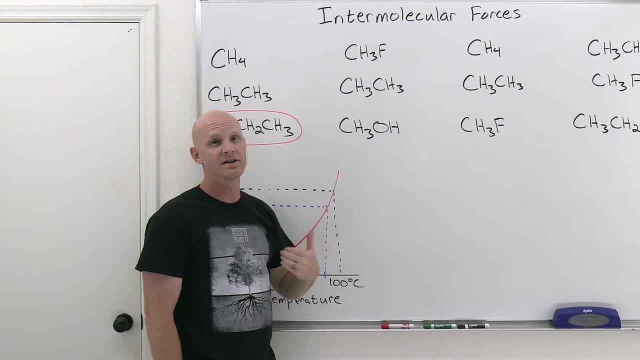 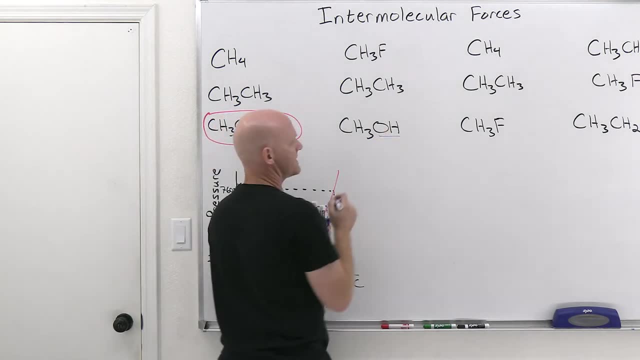 you might notice that he definitely doesn't have any polar bonds and is a nonpolar molecule and all he's got is London dispersion forces. So where it turns out here, you can definitely see that OH bond right there, which means that that molecule is going to have hydrogen bonding. 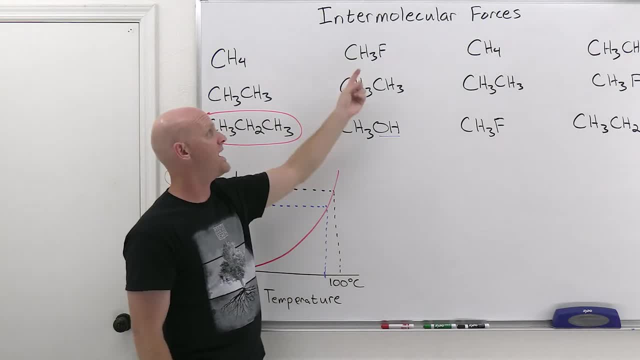 And one of the big mistakes students will make when they see CH3F is they're going to be like, hey, it has H's and F's and it's got hydrogen bonding. No, it doesn't. it turns out If you take a look at the structure. 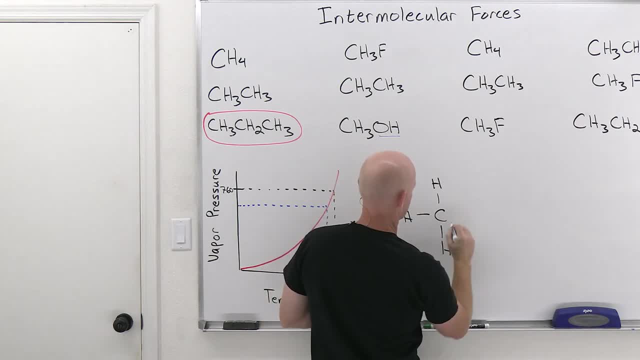 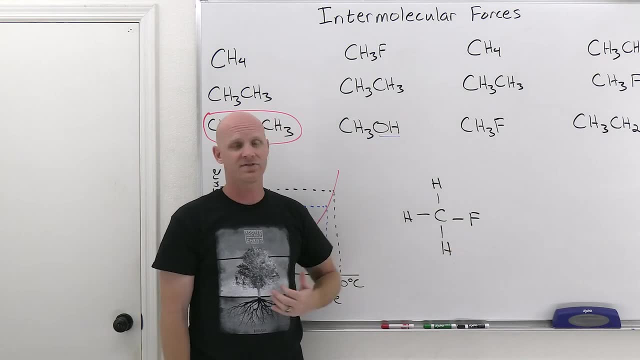 of CH3F. you draw out that Lewis structure, you'll see that even though it does have H's and it does have an F, none of the H's are actually bonded to the fluorine And because that's not the case, there's no hydrogen bonding. 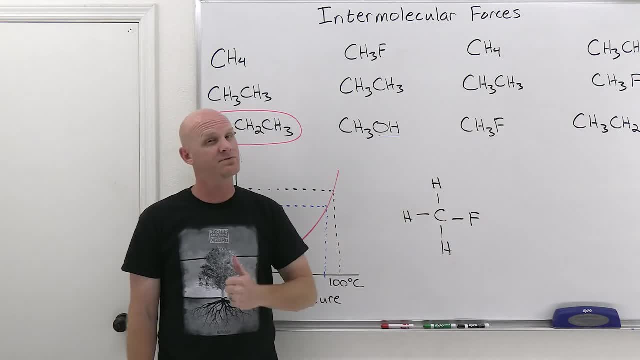 Now it is a polar molecule. There is a permanent dipole here, so it does have dipole-dipole forces, but it does not have hydrogen bonding. Now the reason we're making this comparison between these three is because they're all very similar in size and, again, usually that's going to come. 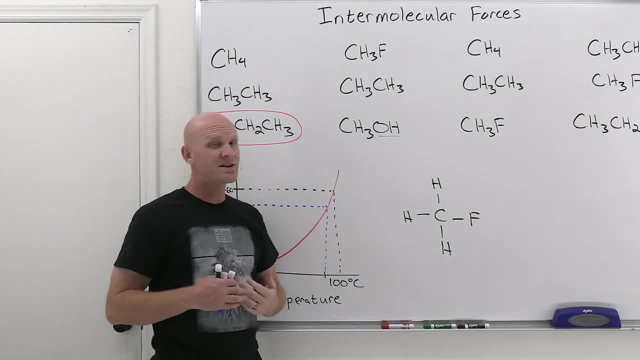 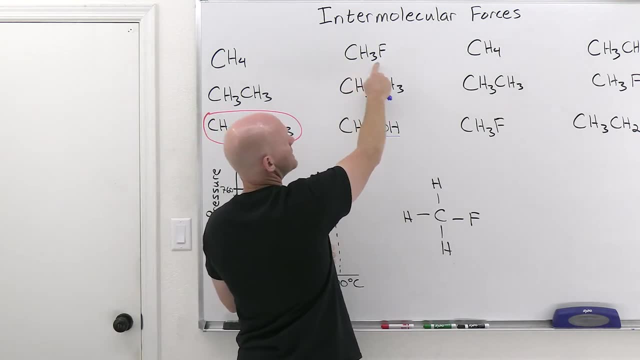 down to, more commonly, molecular weight. but again, surface area technically should play a role. It's just not the one you're most likely to see. So we look at some molecular weights here. So CH3F, carbons, 12,, three hydrons gets you up to 15.. 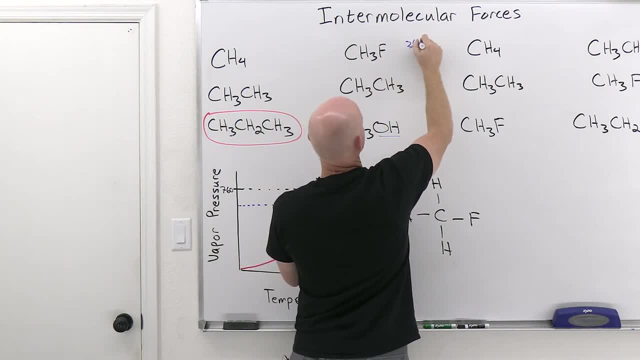 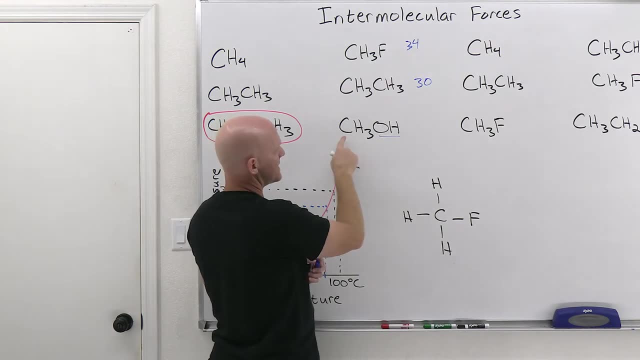 Fluorine here is 19,. so that's going to have a molecular weight of 34.. CH3CH3, that's going to be 15 and 15, that's going to be 30. And then CH3OH- we got carbons- 12, each of the four hydrons gets you up to 16,. 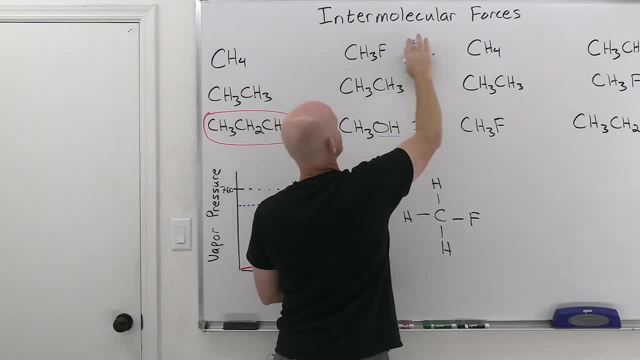 plus another 16 is going to be 32, and let's make this look a little better. So we got molecular weights of 34,, 30, and 32,. they're all very, very close. that are less than 10% apart. 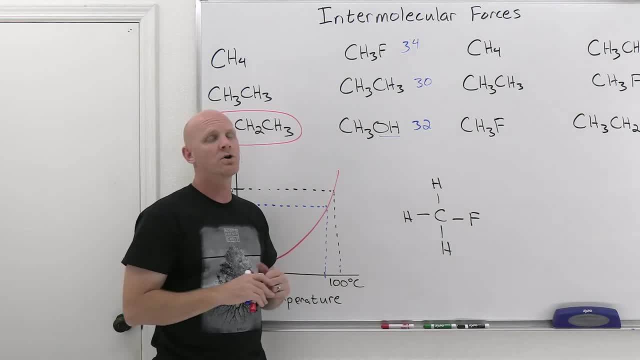 give or take and so being very close. that's again when it's most appropriate to say that London dispersion forces will give the weakest intermolecular forces, then dipole-dipole and then hydrogen bonding the strongest, And since the last one here is the only one of these three with hydrogen bonding. 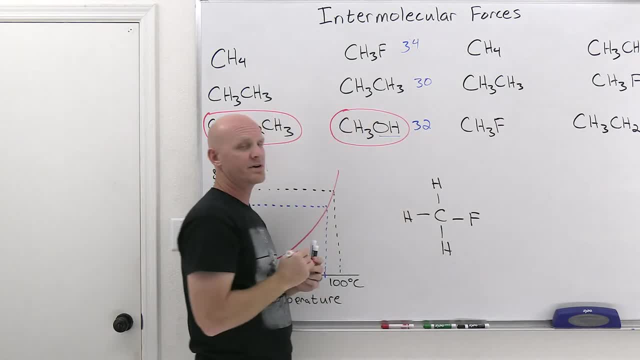 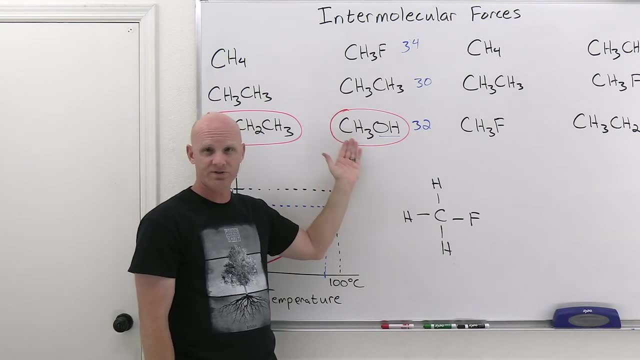 it's going to have the highest or greatest overall intermolecular forces. Cool, and therefore again you'd have the highest boiling point, highest melting point, highest viscosity, highest surface tension, highest chemical temperature and pressure, but lowest vapor pressure. 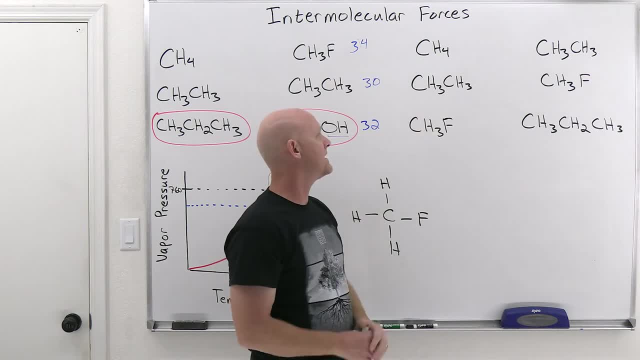 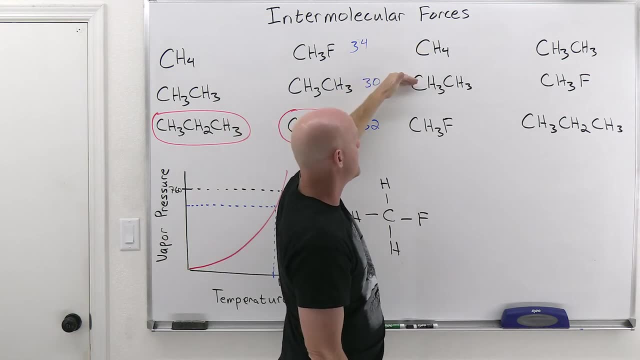 OK, so let's look at this next one here. This next one is going to deal with nobody having hydrogen bonding, So in this case we've got non-polar, non-polar, but polar. So but we should really check our molecular weights real quick. 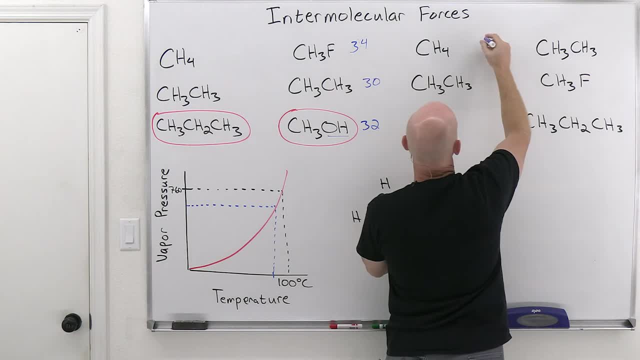 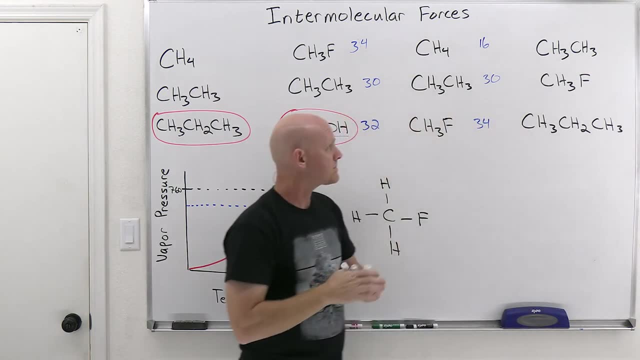 And so we look at the top one. here it's molecular weight, carbon, and four hydrons is just 16,. CH3CH3, we figured out was 30, and then CH3F was 34.. And so in this case, you know, between polar and non-polar. 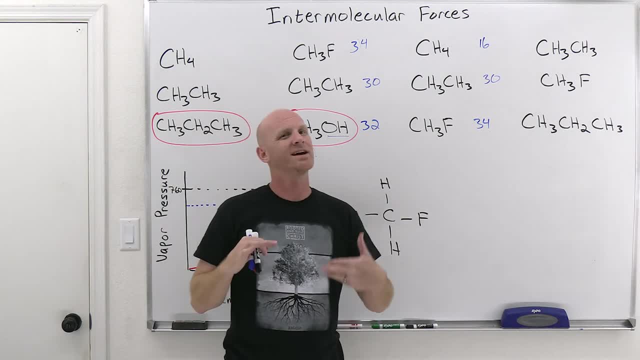 the temptation always: just well, polar, have dipole-dipole and non-polar doesn't. Well again, if they're similar in size, that's the appropriate way to kind of think about it. but if they're not similar in size, we'll find out that's not the best. 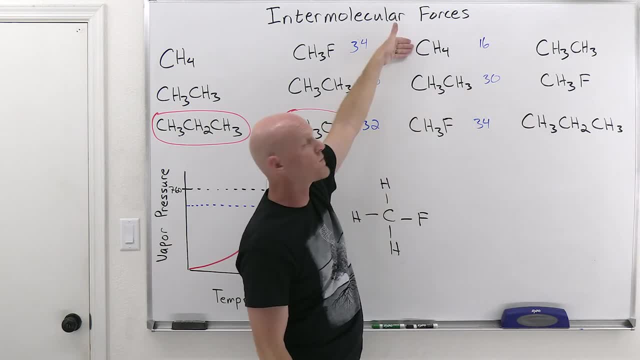 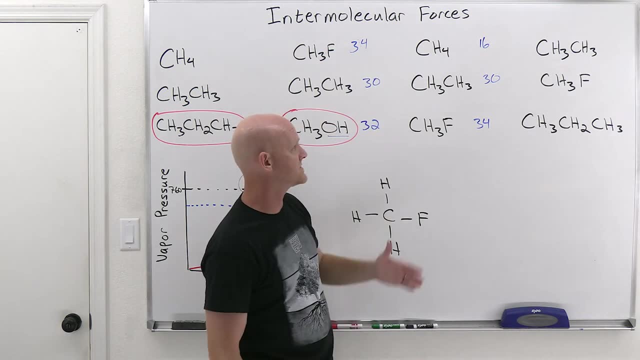 way to think about it. Well, in this case these two are very similar in size, but this one's way smaller And, being way smaller, he's probably just going to have the weakest intermolecular forces, with hydrogen bonding not being something. that's part of the comparison here. 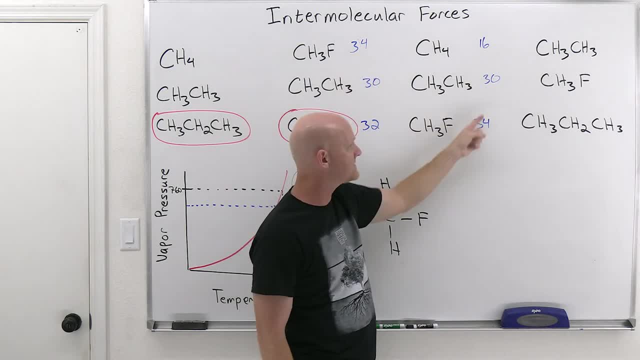 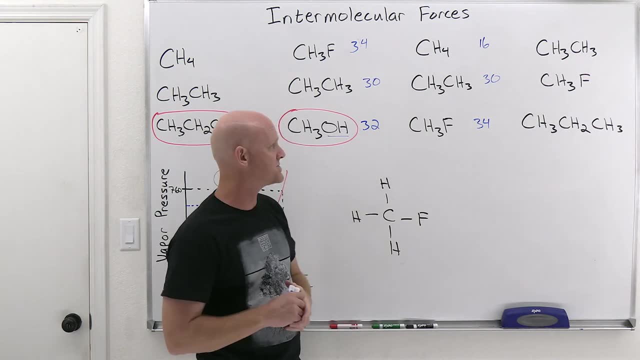 So we'll ignore him. But between these two they are fairly similar in size And by similar here. probably less than like 15% apart is probably what you want to kind of gauge by, And so in this case then it really is going to come down. 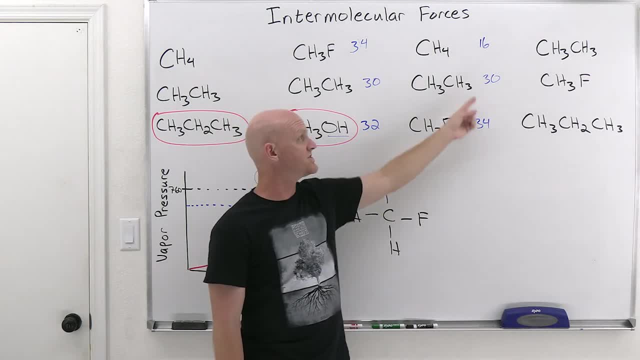 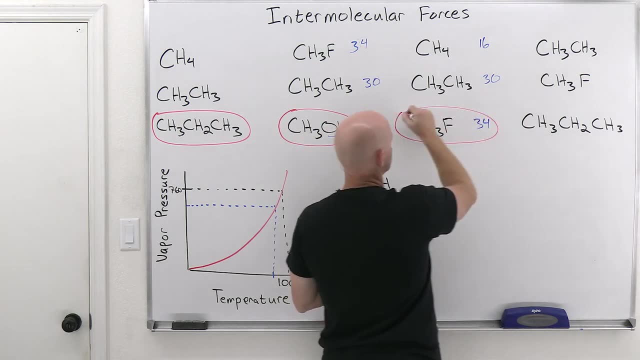 to dipole-dipole forces, which he has and he doesn't, And so not only is this one just a little bit bigger, but he also has the one that has the dipole-dipole forces, And so he's going to have the overall greatest intermolecular forces. 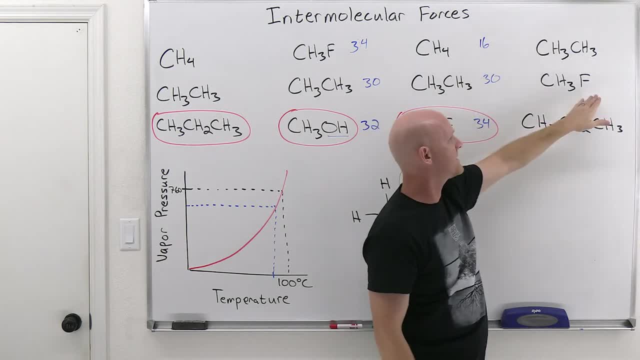 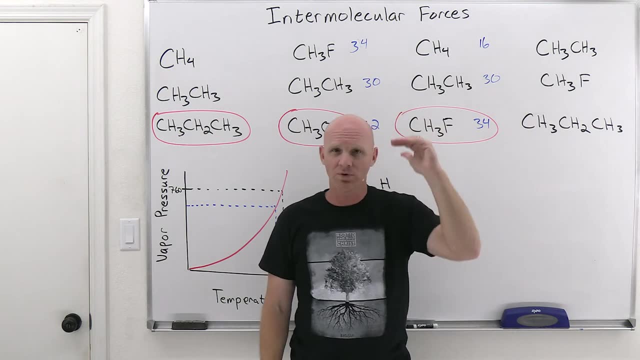 All right. so this last comparison: we've got two that are non-polar, one that is polar. we still have no hydrogen bonding on the table. So and again, the temptation is just to pick the polar one, But again, dipole-dipole is stronger. 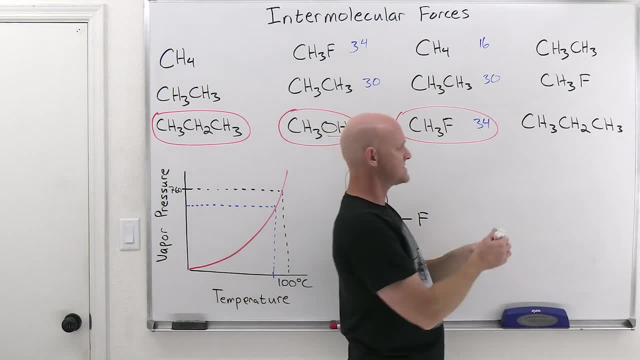 than London dispersion if they are very similar in size. So let's take a look at our similarity in size here And again. CH3CH3- we've done a couple of times. It has a molecular weight of 30.. CH3F- we've done a couple of times. 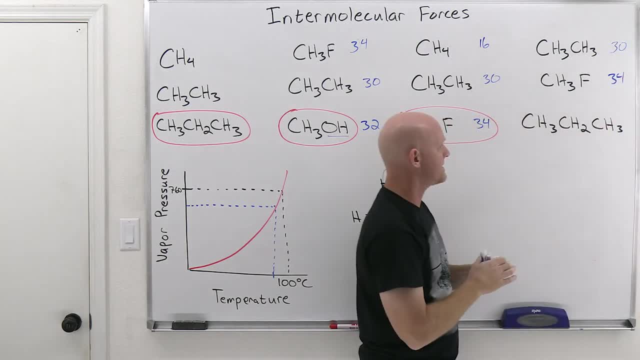 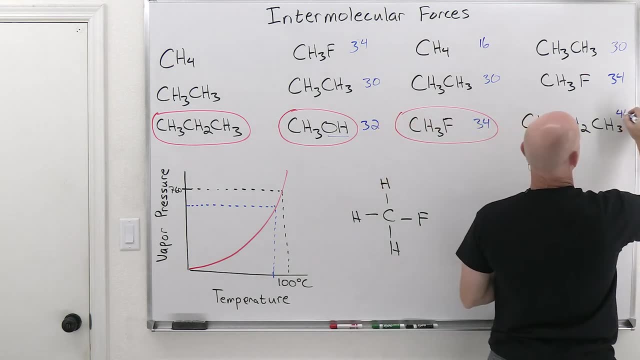 A molecular weight of 34.. However, this last one here has got three carbons, That's three times 1236, and then eight hydrons. So add another eight and you're going to get 44. And so now, all of a sudden, you know 44 compared to 34.. 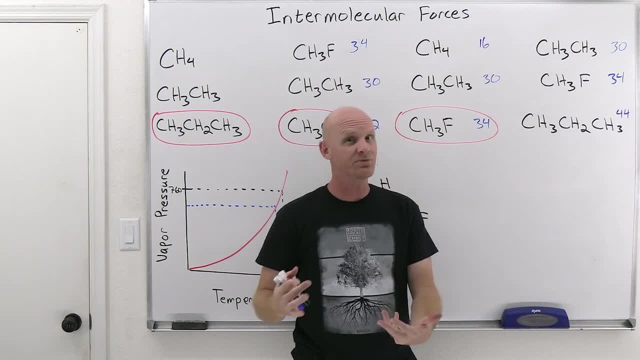 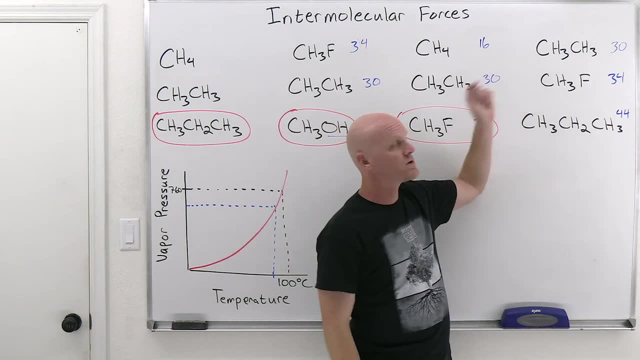 That's almost you know. an additional third, additional 33 or 33 percent or so. That's a substantial difference, not just, like you know, 10 or 15 percent, It's like 33 percent bigger than this one right here. 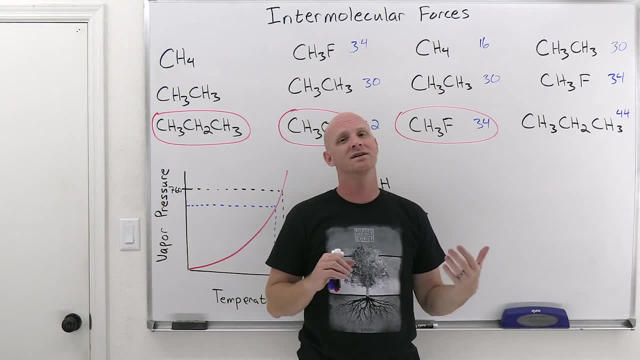 And when that's the case, if they're not pretty darn close in size, then all of a sudden you know it won't matter if one's got dipole-dipole and one doesn't, the bigger one's going to have enough extra. 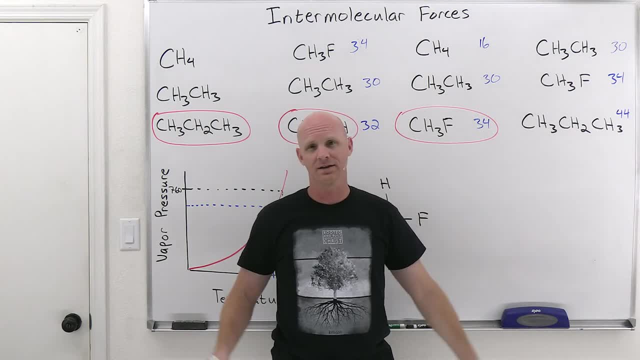 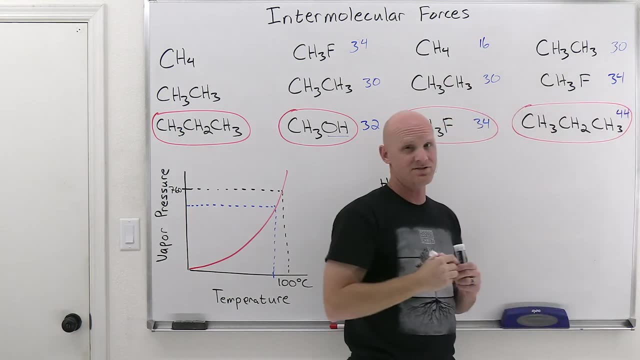 London dispersion forces, whether it's the polar one or not, to overcome any difference in dipole-dipole forces. And so it turns out this last one actually has the greatest overall intermolecular forces out of these Three. So notice the difference between these last two sets. 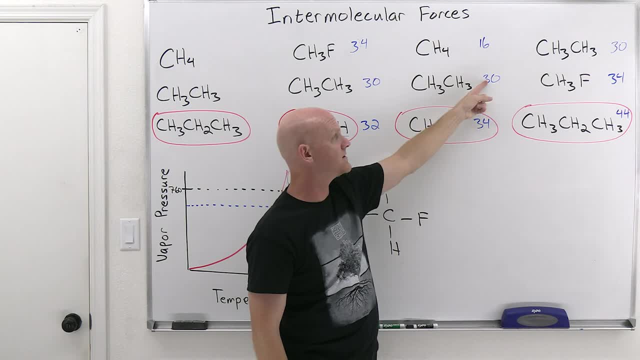 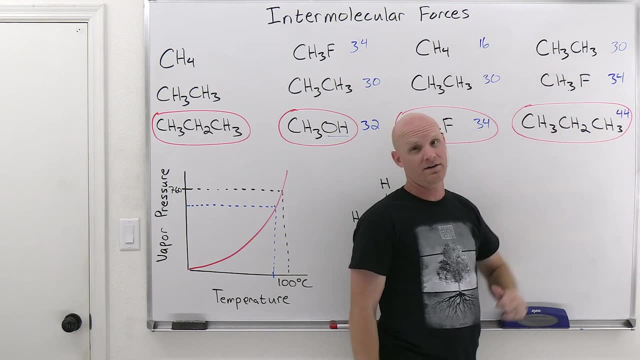 So here we compared a polar and a nonpolar that were very close in size, just a little over 10 percent apart. But here we compared a polar and a nonpolar that were now, you know, like 25 to 33 percent apart. 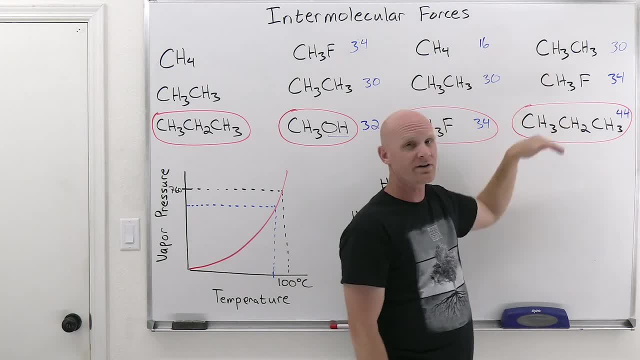 a much more significant difference And all of a sudden it was not going to be a fair comparison. You know we can't say, all things being equal, dipole-dipole stronger than London dispersion, because all things aren't equal. So the increase in size or the 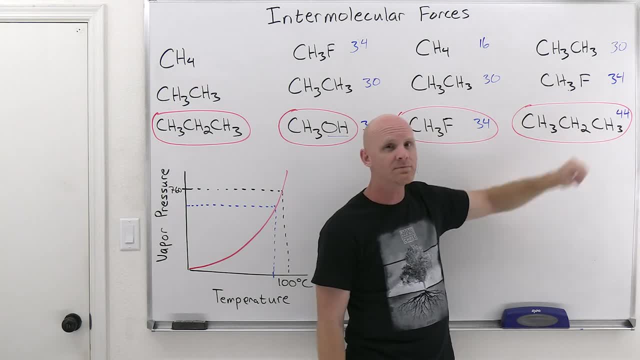 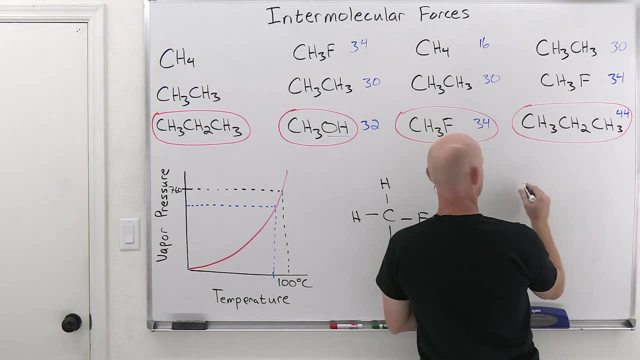 the greater. the size in this one compared to the polar one was more than enough to make up for that. So I just want to point that out Now. if you know, the comparison I made was say this one right here: 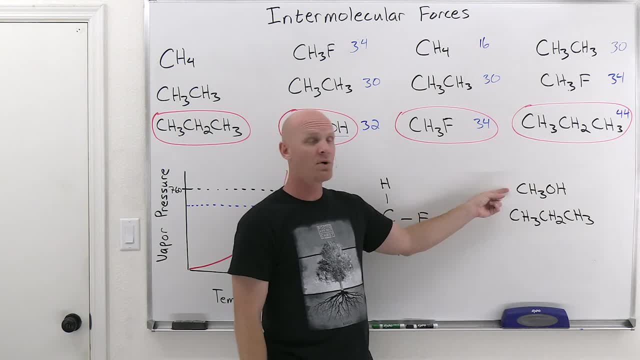 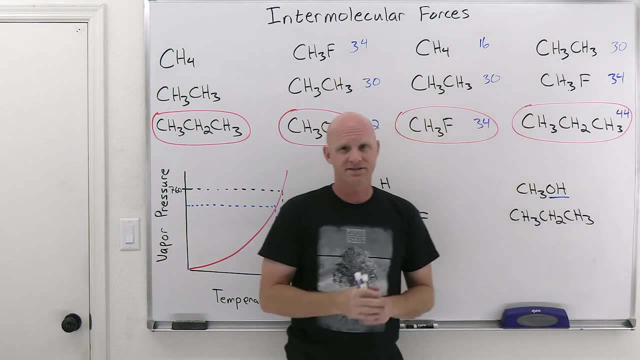 Well, again now I have a nonpolar one that's bigger, and then I have a polar one that's smaller, but not just polar, polar and having hydrogen bonding. Now it turns out, you know, this guy to you know be bigger than a polar one. 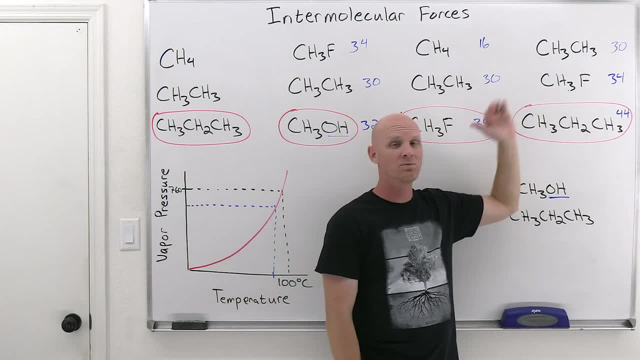 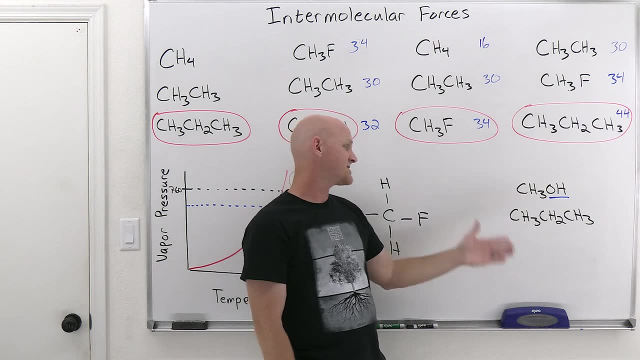 and have the higher overall intermolecular forces. he just had to be, like you know, more than 15 percent bigger in size But to overcome hydrogen bonding, which is significantly greater in strength. all of a sudden, now it turns out in this comparison. 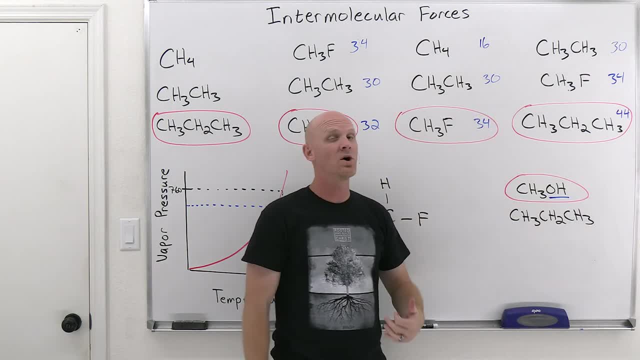 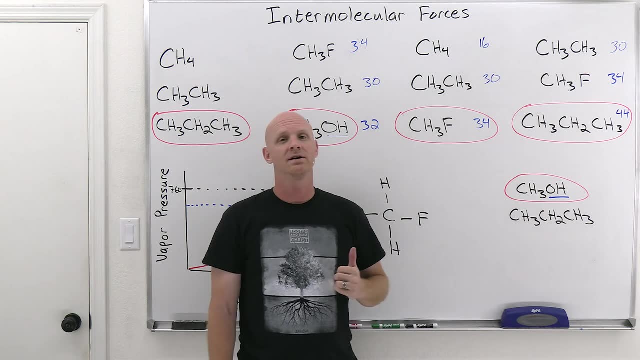 he's going to have the greater intermolecular forces between these two, even though he's smaller. So when hydrogen bonding is on the table, that's usually going to be king. Now, can I make a nonpolar molecule big enough so that it's even you know? 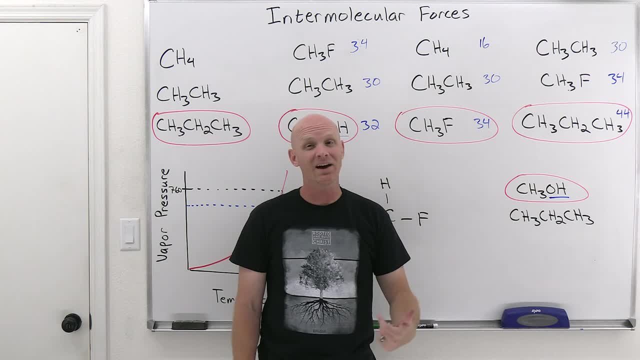 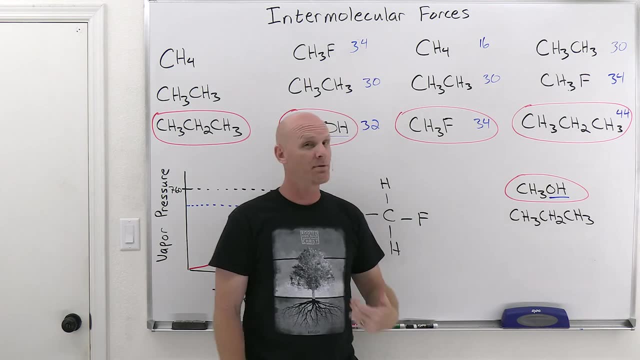 has even greater intermolecular forces than, say, something with hydrogen bonding. Well, I can, but it's not just like a little bit bigger. It's probably going to have to be, like you know, 100 percent bigger or something like double the size, bare minimum or something. 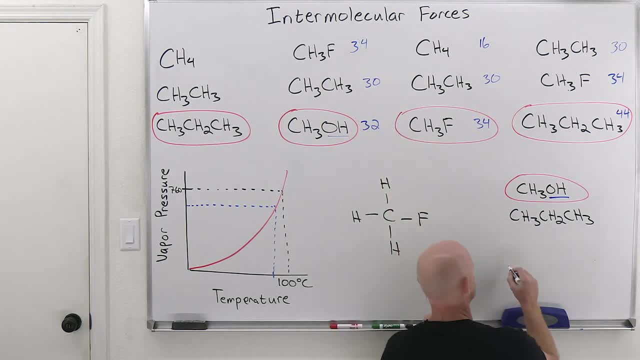 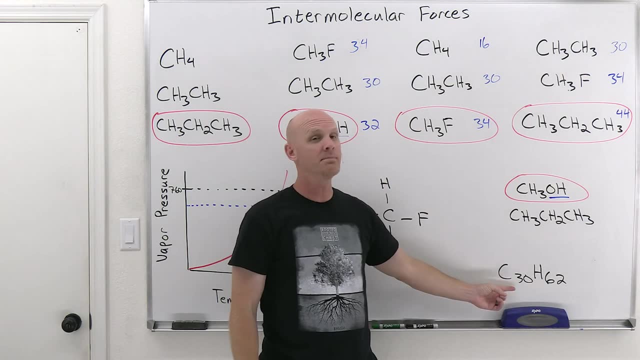 like this. Now, the truth is, I could give you something, like you know, C30H62 or some giant structure, And this is now going to have a much higher overall intermolecular forces than, say, this guy which has hydrogen bonding. 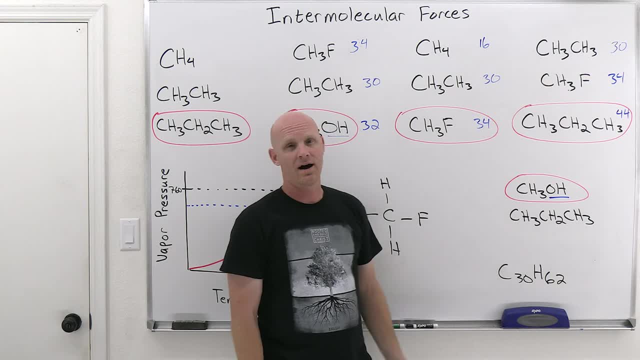 But notice it's significantly bigger. This thing is huge And this would be an example of something like a wax or something like that. It is nonpolar, but it's actually got such high intermolecular forces that it's a solid at room temperature. 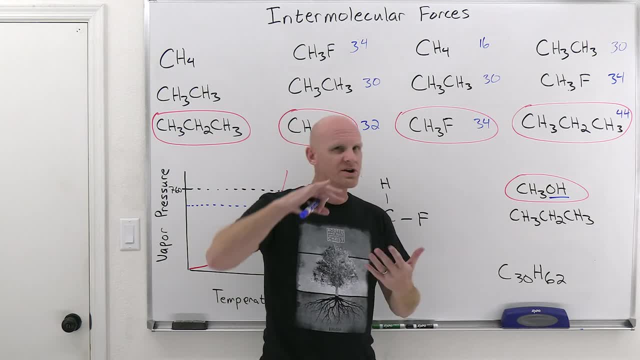 So it is possible, but it's also very difficult, Like what's the threshold, And that's something that you're not as likely to be quizzed on, So I do want to make you aware of the fact that it is possible. 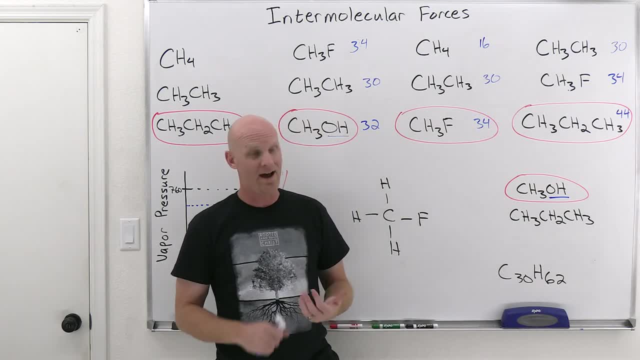 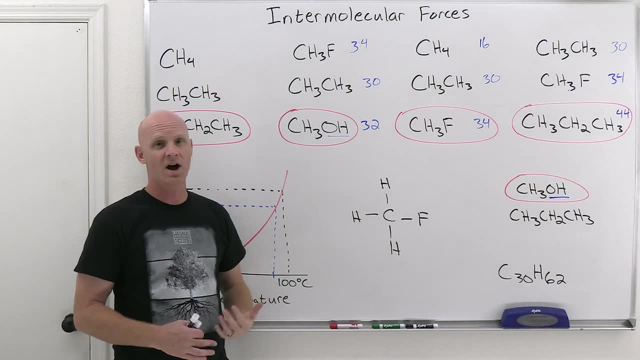 but it is not something they're likely to encounter on a general chemistry test. So if you've got hydrogen bonding on the table, hydrogen bonding is usually going to rule the day whether there's a difference in size or not. But if there's no, 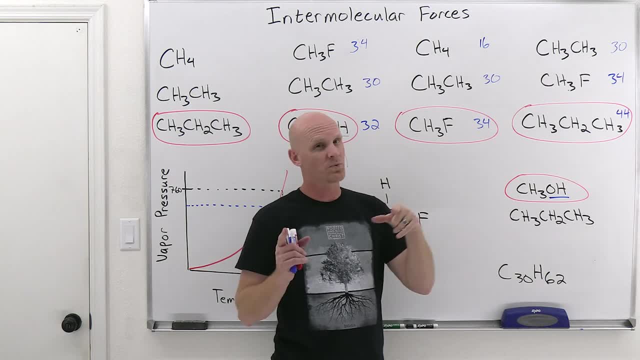 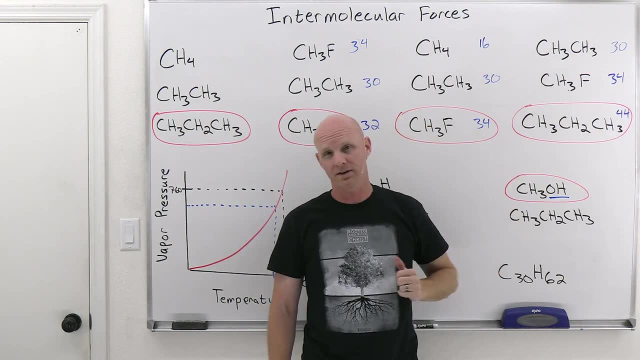 hydrogen bonding on the table and you've got some that are polar and some that are nonpolar. it really will come down to: are they very similar in size? Then go with the polar one. Are they not similar in size? Then go with the biggest one to have the overall greatest intermolecular forces. 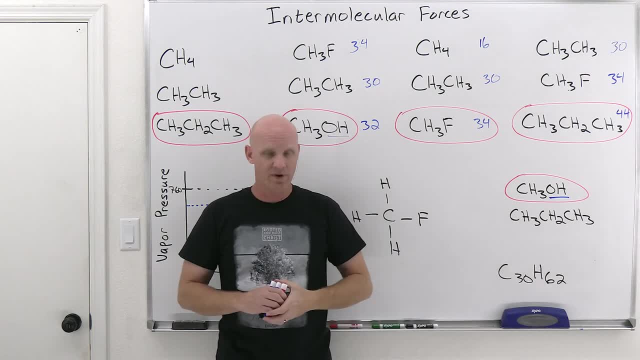 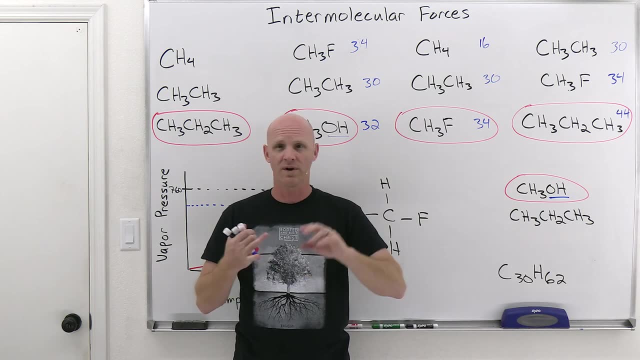 Cool, And that's really what it comes down to with intermolecular forces And you want to get good at recognizing all the intermolecular forces present and which has the greatest or lowest and how that affects those bulk properties If you're ranking boiling points or 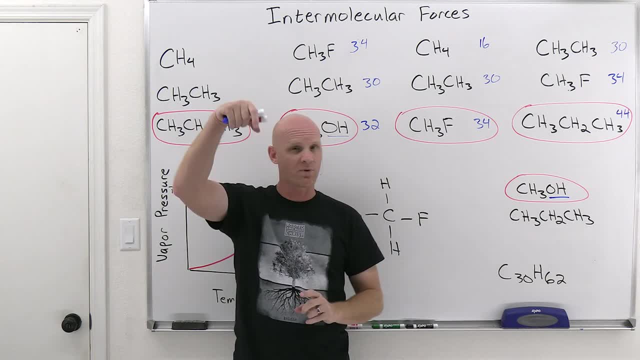 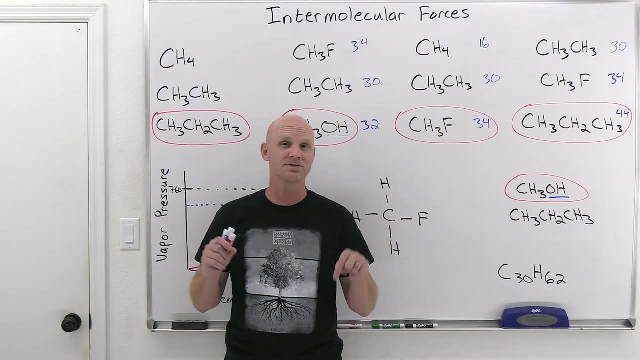 surface tensions or viscosities or things of that sort. And again, don't forget that vapor pressure goes the opposite direction. Now, if you found this lesson helpful and you want to support the channel, a like goes a long way to making sure other students get shown this lesson.